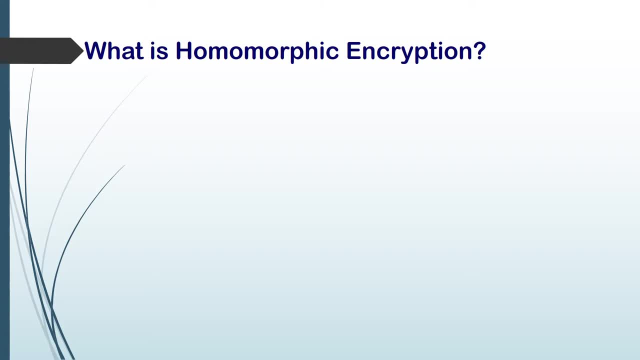 The inputs of our particular data. That is what every bit simple called encryption. But when we say homomorphic encryption, it's not that we are doing encryption on numbers, but instead, in homomorphic encryption, we are focusing on the encryption of ciphers. ciphers a data different from numbers. 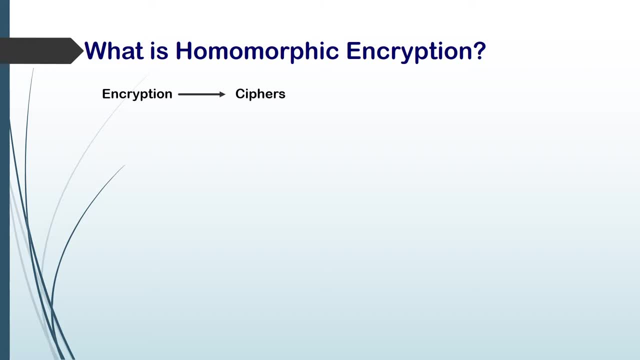 and character ciphers that are a bit more complex than numbers and characters. Similarly, we will see that homomorphic encryption is a part of a crypto system, and by crypto system we mean that it composes of cryptographic algorithms. this is also a very broad term. it can be defined in: 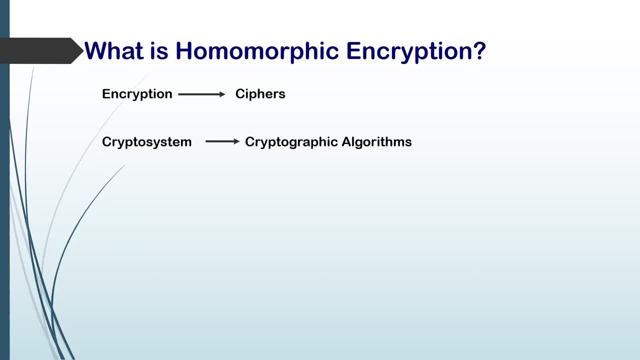 many ways, as the user wants, but in simple we will say that homomorphic encryption is a type of a crypto system. and what is a crypto system? crypto system is basically any type of system, is any algorithm which runs cryptographic algorithms. but what is the goal of a crypto system, the goal of 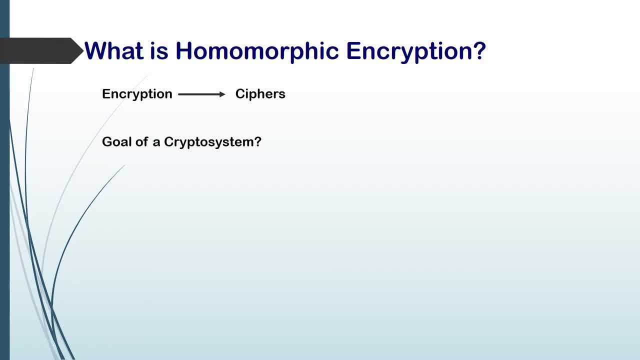 the crypto system is basically what we can say, the goal of overall cyber security, because homomorphic impression is basically a subset of cyber security field. so the goal of the cyber security, you can also call it as the goal of homomorphic encryption. but what is the goal of cyber security field? 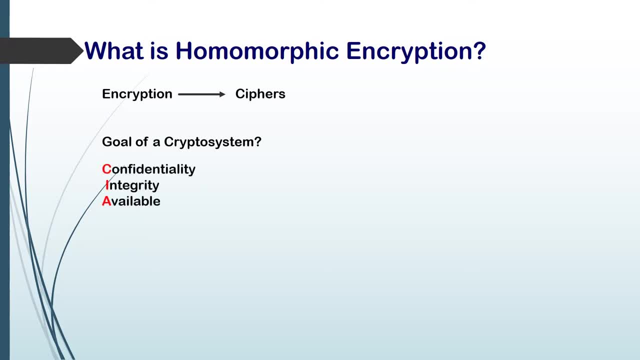 basically, cyber security field comprises of three things: confidentiality, integrity and available. this is what we call, in simple words, the cia of cyber security. similarly, we can, or in other words, we can also say that these three things are the main objective, these are the main purpose of performing. 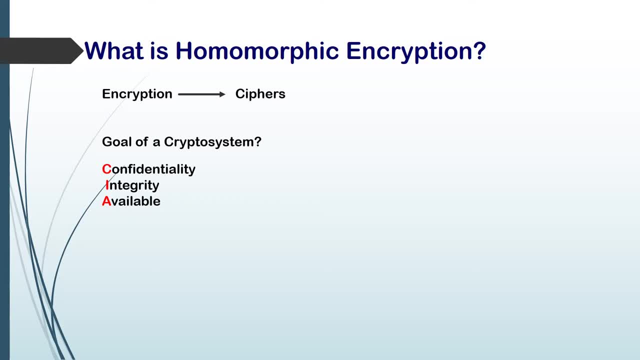 homomorphic encryption on some particular data. now let's focus on a simple model of homomorphic encryption. for example, we say that a user has some data- now the data of the user- we will perform a process called encryption. encryption is somehow messing with the user data in a particular way that it can be forward. 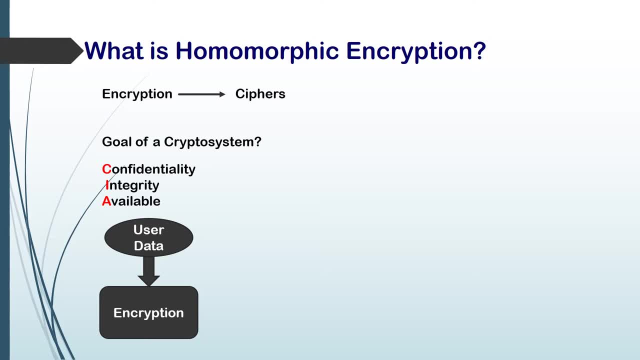 that it can be forwarded back. it can be reversed. now, with this encryption, as on the in data, we will obtain something called encryption encryption. as on the in data, we will obtain something called encrypted data. that encrypted data will then be sent on to the public internet, or in particular, for instance- let us say that it is sent. 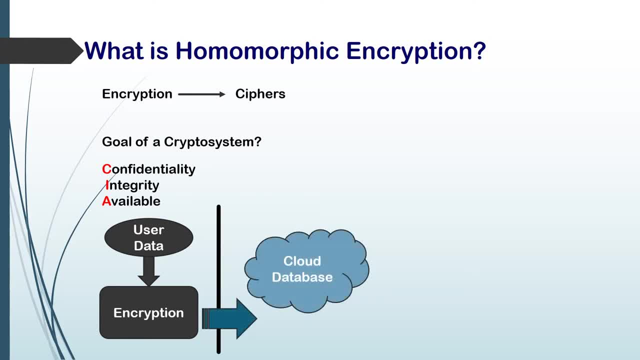 to a cloud database. the cloud database is something that belongs to a specific company. it belongs to a remote server. now this particular cloud data will perform, let's say, any computation on data, but on encrypted data instead of the original plain text data. now this encrypted data, let's say, is going. 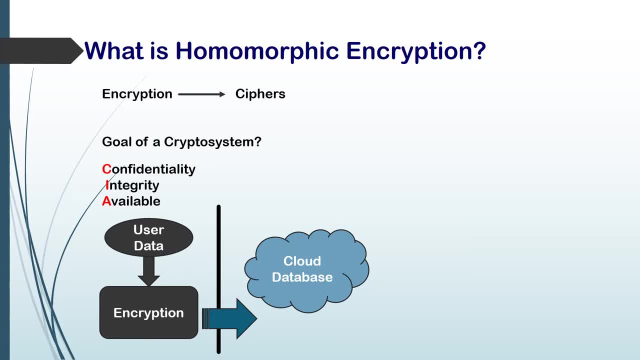 to be accessed by another user, located at any other part of the world, in order to operate any computation on the data. if computations are performed on plain text data, then it will be the violation of the privacy of the first and user. first and user. so what do we do? we say, for instance, that we want to send data to a trusted 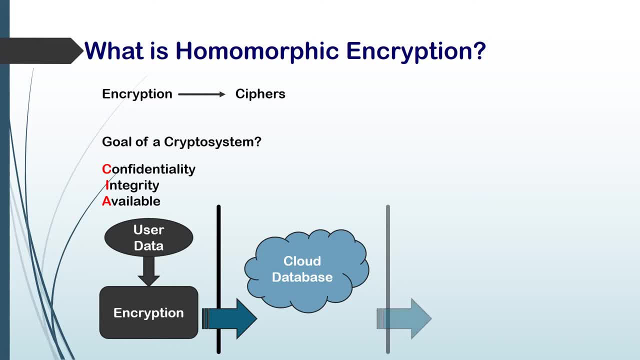 end user to perform that operation. we perform assist, we perform a system, a process called as decryption. decryption is basically the the reverse back method of encryption. we have some cipher text, we have some encrypted data. we perform decryption. decryption converts those cipher texts back into plain data text. 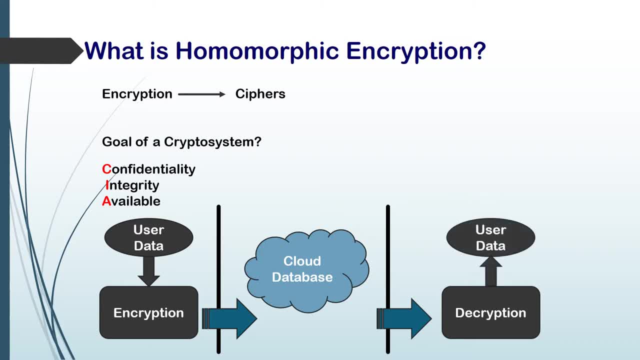 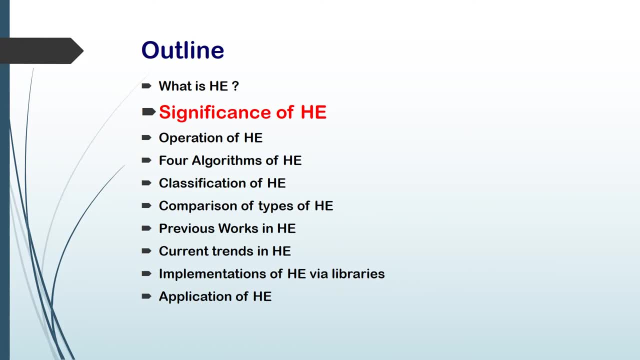 and that plain data text is then delivered to the end user. now let's see the significance of homomorphic encryption. why is it so important in today's society, as we know today, that more and more users are connecting to the internet? more and more devices are being increased, either in the form of smartphones, 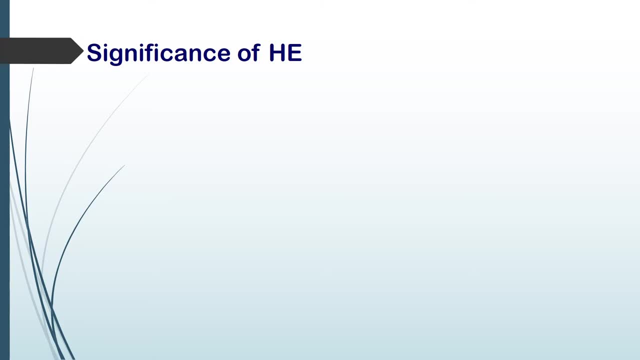 they are in the form of tablets, laptops, computers, servers, any end system. more and more devices are increasing on the internet, which ultimately means that we need to devise a method to protect data of these individual devices, of these individual nodes, or in other words, i can say that online data 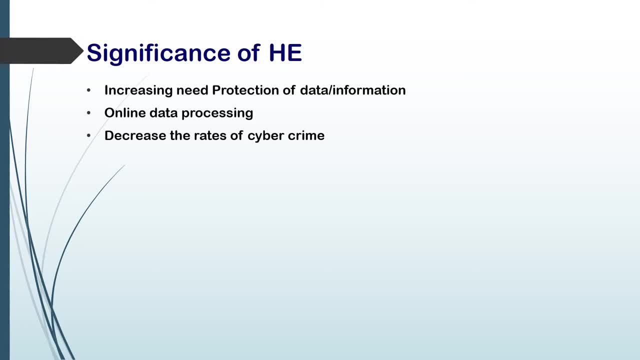 processing is increasing. online data processing is increasing. this has an ultimate effect on the privacy of the data of the end user. if we perform data processing on the directly on a plain text of an end user, it it violates the cia of homomorphic encryption. similarly, in order to prevent 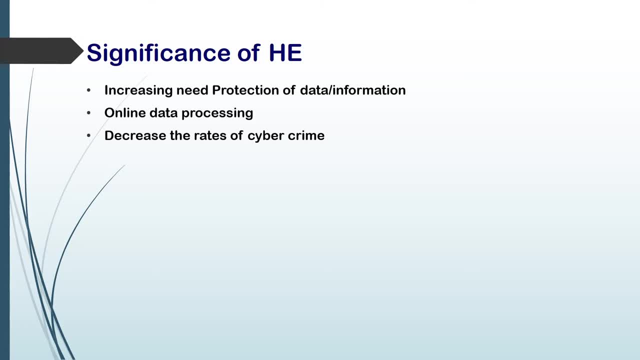 all of this. we need to devise a method to protect these data. we need to decrease the rate of the cyber crime occurring all over the world. this is why we need homomorphic encryption. but why do we need homomorphic encryption instead of encryption? we will discuss in a second that. why is homomorphic? 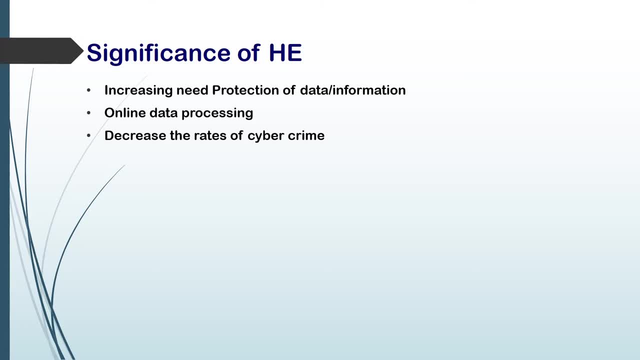 encryption more important as compared to simple standard encryption. first, let us discuss a few examples of where homomorphic encryption could be applied. we will discuss a few examples- few hacking examples that were hacked previously. first of all, we would like to discuss the very famous sony playstation 2011 hack. this was one of the most violent attacks that ever occurred. 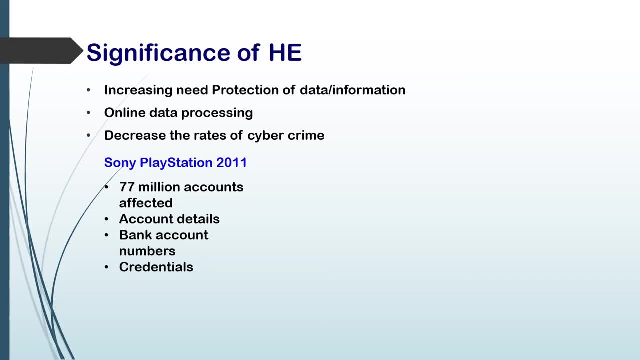 including 77 accounts were affected. the account details were stolen, the bank account numbers were stolen and, similarly, the conditioners were also stolen. this is a very huge and major attack that ever occurred. similarly, another attack also occurred on equifax in 2007.. 143 million accounts were directly or indirectly. 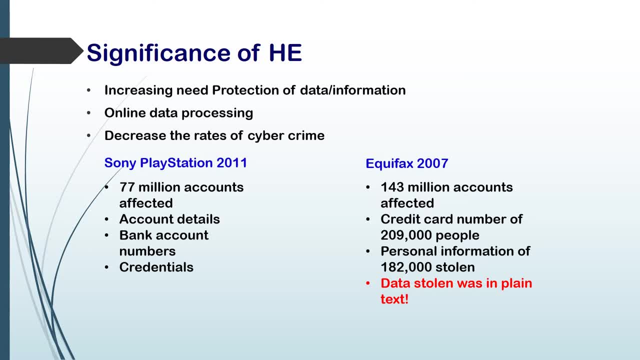 affected the credit card numbers of two hundred and nine thousand people. they were stolen or either corrupted or either sold out on the black market. personal information was also sold and, the most important part, the data stolen was in plain text. they didn't have any type of protection. they didn't have any. 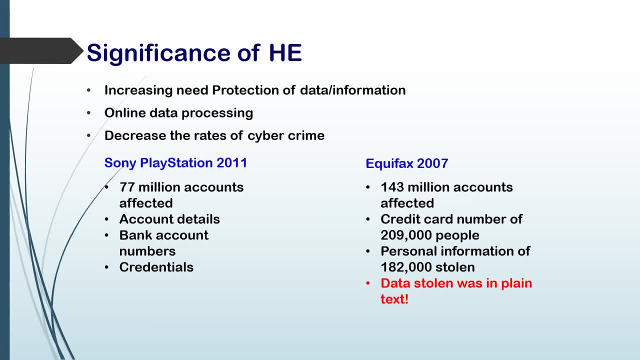 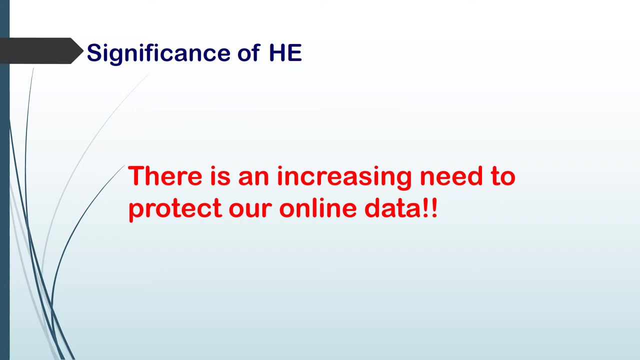 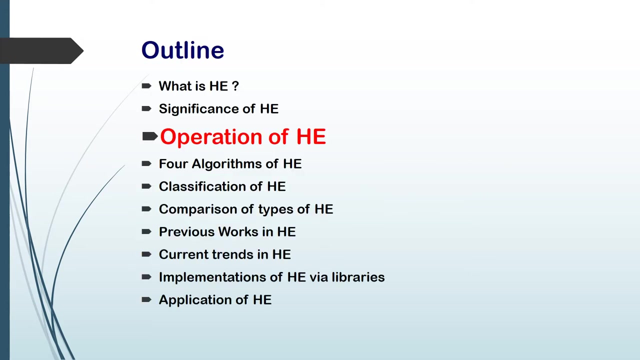 type of encryption to do on the users data in order to protect it, but instead the data was stolen. in the plain text, this is a major breakthrough. this is a major problem that occurs in cybersecurity. therefore, there is a major need to protect our online data. next, we will discuss the operation of homomorphic encryption. 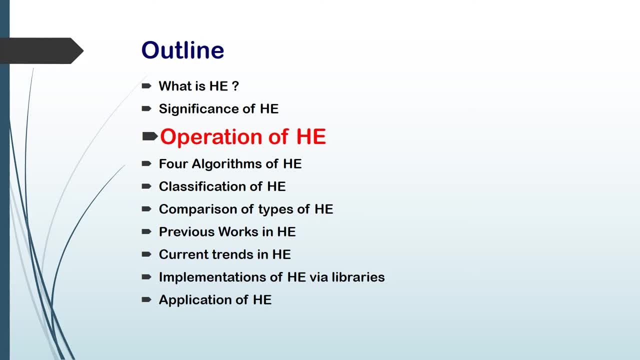 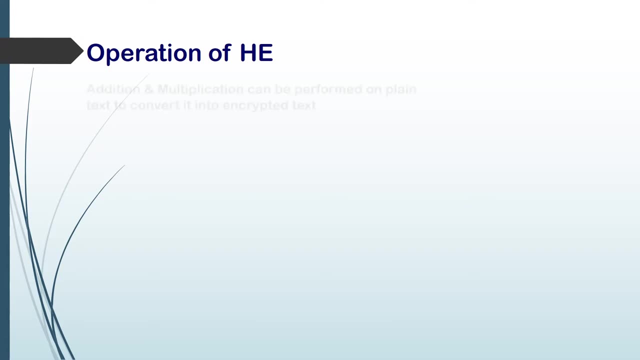 basically how it works. to start with, homomorphic encryption basically occurs at a very individual, at a very basic level. we can say that homomorphic encryption either occurs in the form of addition or it occurs in the form of multiplication. but why am i saying this? because when we practically implement homomorphic encryption, they 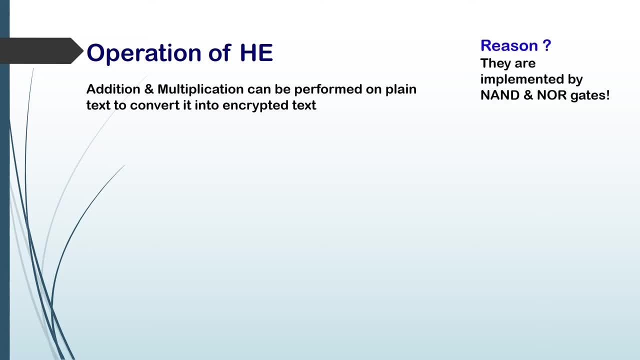 implemented either in the form of NAND gates or either in the form of NOR gates, because these two gates can be used to apply the operation of addition or multiplication. now I would like to discuss a very compact example here on what do i mean by addition and multiplication in the context of 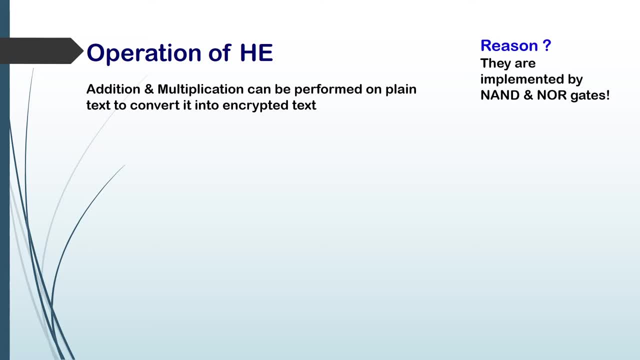 homomorphic encryption. let's say that i have two numbers, two and four, and I want to perform some type of encryption on them. that encryption, let's say, is a function which doubles the input that I gave it: 2 is doubled to produce 4, and 4 is doubled to produce 8.. 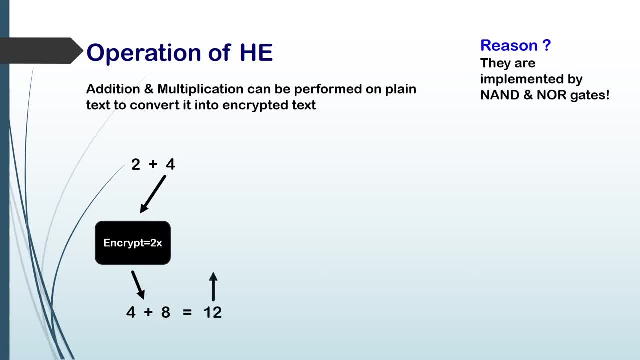 This produces a result of 12, and this 12 is then decrypted back into 6.. Now, in this manner, 2 plus 4 is equal to 6.. Let's say that this data is called the plain data. This is what the user produces, and encryption and decryption functions are basically the homomorphic encrypted 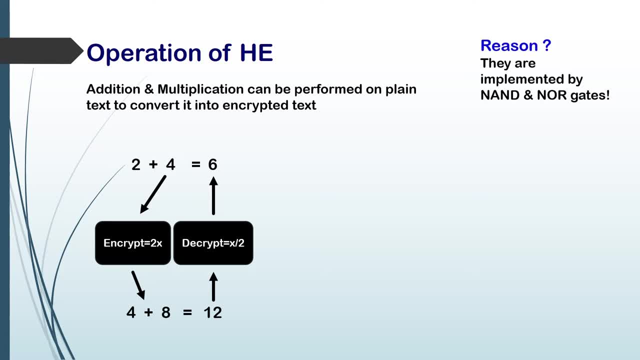 functions they perform the operations on these plain text data. 4 plus 8 is equal to 12.. This is the encrypted data that is produced after the encryption, or we can called this data as the ciphertext data. This is the data that practically goes on the internet Goes. 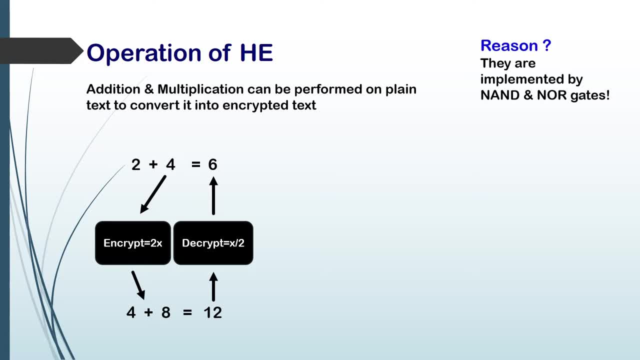 on the cloud And computations or operations are performed on this type of data rather than the plaintext. this type of encryption is called as additive homomorphic encryption because it uses the operation of addition to perform homomorphic encryption. similarly, as we can all guess that multiplication, or multiplicative HE, is also similar to. 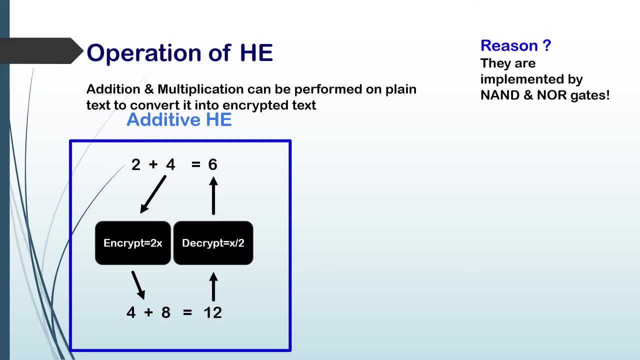 this very additive HE. instead of using addition, we are using multiplication. we have two inputs, they are encrypted and operation is performed to produce a result. in this case, the result is 16. 16 is decrypted back to produce the plaintext form of 8. similarly, this is called multiplicative HE. this is a 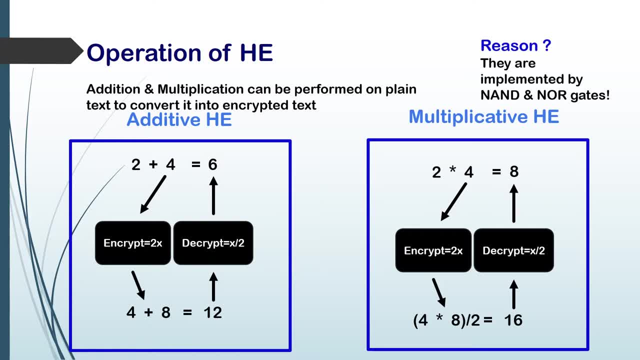 bit more complex method of decryption if we want to add a version of this to a operation of homomorphic encryption. other homomorphic encryption that we will discuss later are based on this same principle, but at a very, very large scale. next we will see that they are basically they are four algorithms. they 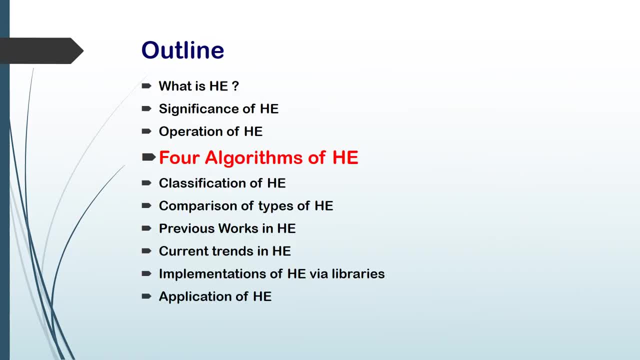 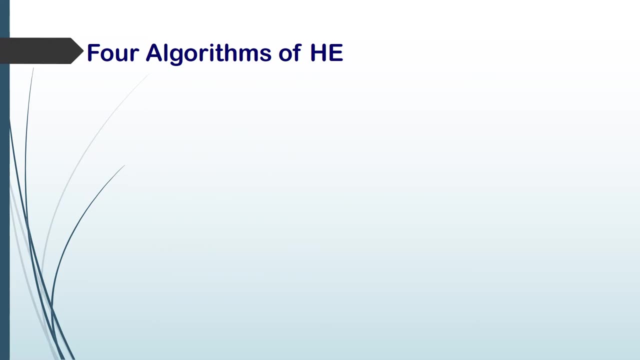 are operating in the context of homomorphic encryption. therefore, algorithms are also based on the operation that we just discussed, but in a more compact way. the first of the four is called, let's say, the encryption method. I can say the key generation method. in the key generation method, I say that we 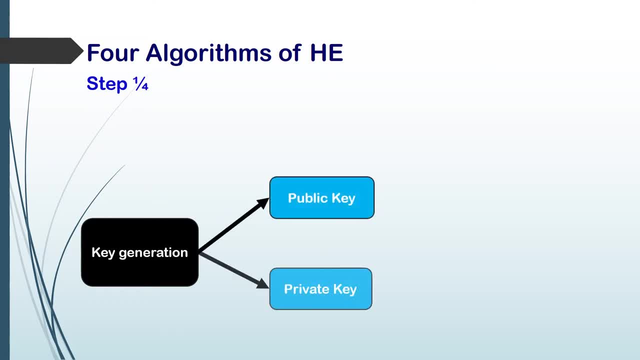 produce either a public key or a private key. now, these are two different things. these are recently to develop new things. what I mean by a public key? let's say that I encrypt my data and I want to send it on the cloud, for instance. let's say that I have a public key and I want to send it on the cloud, for instance. 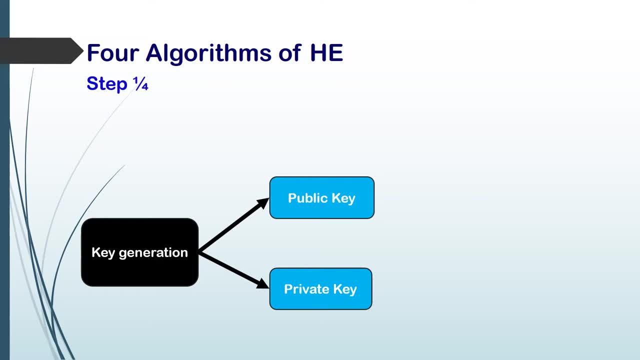 some data and i have copied my data onto my dropbox account, for instance. and dropbox, for instance, let's say, wants to produce any type of computation, it wants to produce any type of operation on my data. so what it will do, it will produce an encryption, it will produce an. 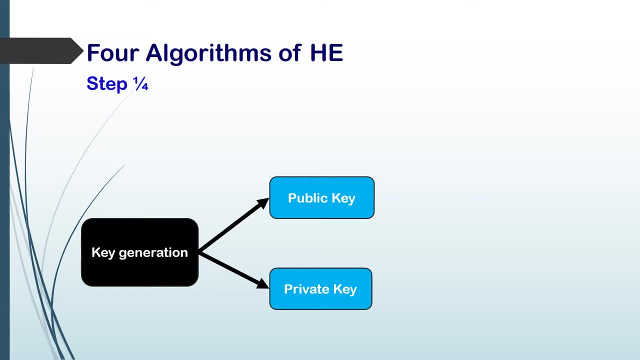 encrypted data using a public key. so a public key is a sort of encryption key. when performed on data, it produces the result which can then be processed into the public. this is what we call a public key. and now, as we can guess, private key is another different thing. private key is when, for example, 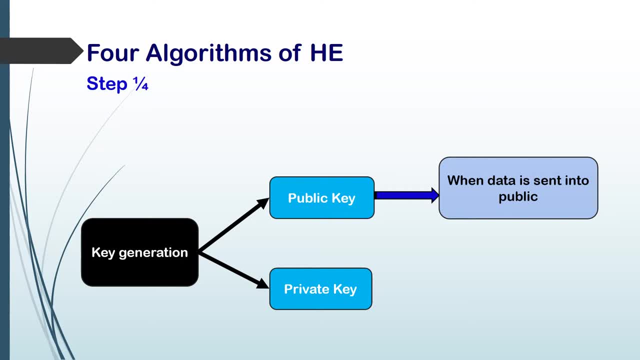 an end user wants to access that data. let's say that i want to access my data. back dropbox will send me my data in encrypted form, in cipher text form, and then I will have the private key in order to decrypt my data. This is why we called it is a private key, because it can only be used by the end user. 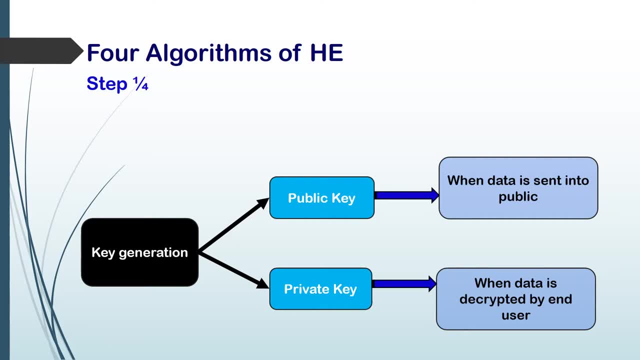 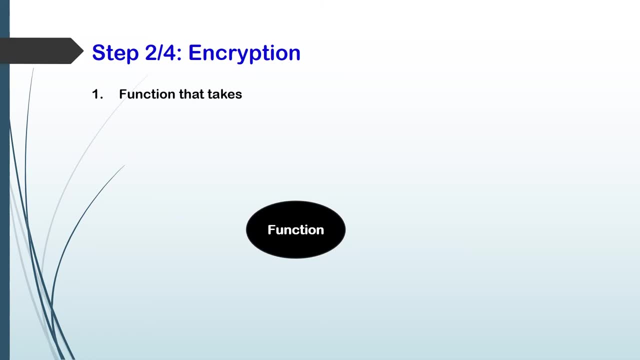 Now the next is what we call an encryption function. In encryption function, we say that we have a, basically a function. It takes two inputs: the first, plain text, as we discussed before, and the second it takes public or private key, depending upon the encryption you are going to perform. and now it performs. 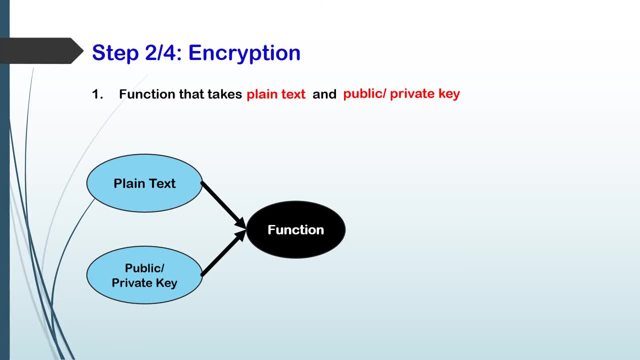 any operation. but in this context, let's say that it performs the addition operation. It adds both of them, then it generates something called as encrypted data in encrypted form. or we can say that it performs The cipher text. it generates the cipher text. Next, after, after, encryption, we can see that the most important is decryption. 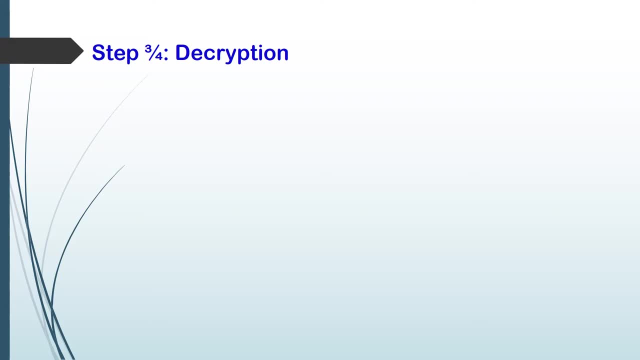 Now we have generated the cipher text, we have generated the necessary matched up version of our data. Next we will do the decryption. we will convert that matched data back into the original form. Similarly, we will have a function. the function will take two values. first of all, the cipher. 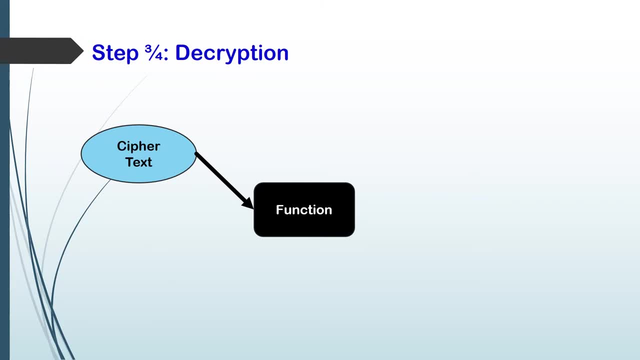 text. The cipher text is the same grumbled up text of our input and the second input it will take is called private key. because private key we are using in this case? because an end user wants to have access to the encrypted data. that is why we are using private key. 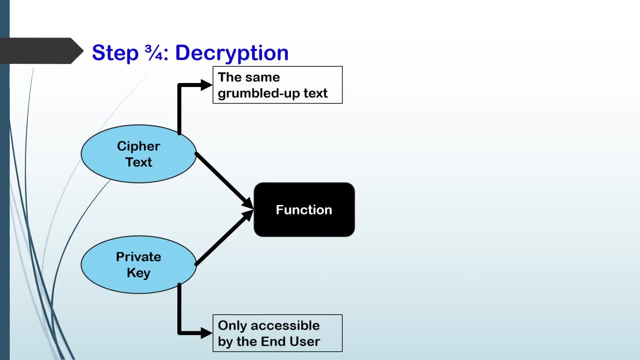 here- and this is only accessible by the end user- and that function, whatever it performs if addition, it will perform similarly a similar something to addition. in case of multiplication, It will perform the opposite of multiplication and it will produce some useful data. Now, step 3 was about performing the cipher text, performing the operation on the cipher. 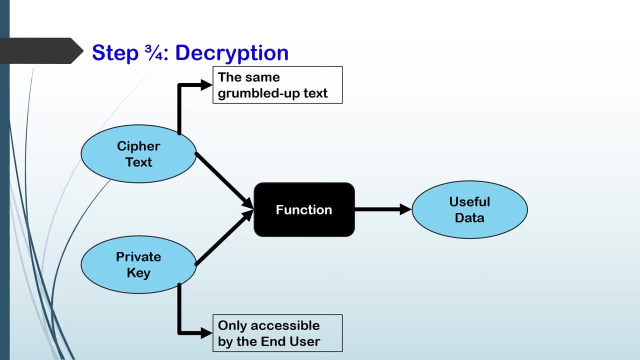 text, either on the end user. the end user wanted to gain access to the data. that is why we use the private key, but let's say that our data wants to be processed in the public. This is where step 4 comes in: the evaluation or the processing of the data. this is the 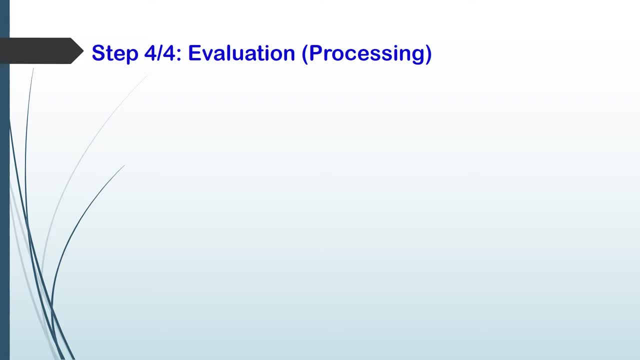 most core part of the homomorphic Okay encryption. this is where we perform operations, we perform competitions on our encrypted data, on our ciphertext data. this is as we discussed. this is one of the core parts of HE. this is performed in the cloud and any third. 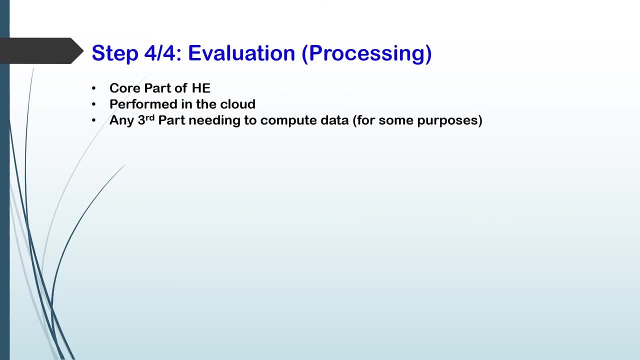 party needed to compute data for some purposes. for some purposes, but remember that data is already encrypted with a public key and computation is performed on the encrypted data, which means that the user, the party, that whoever party is performing an operation on the ciphertext data, he does not have access to the 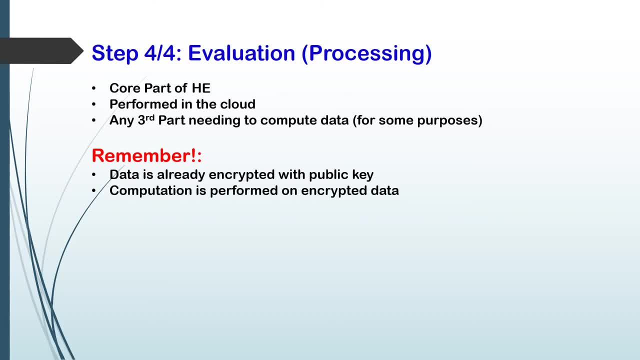 original plain text data. this is why we use homomorphic encryption instead of standard encryption, because in homomorphic encryption we have data on. we have data in the form of encryption encryption. we have encrypted data. whoever wants to perform any type of operations will have to deal with the encrypted. 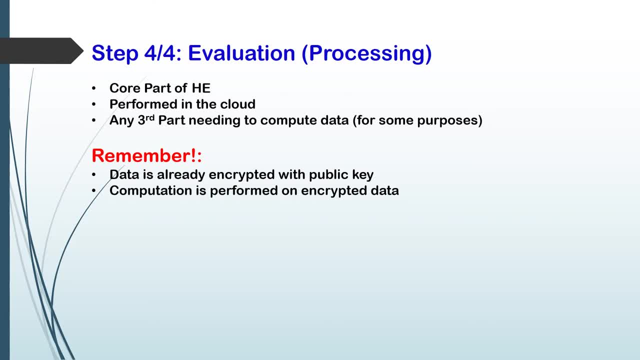 form. now some additional operations, some additional actions which can also be performed on homomorphic encryptions. are these: data is somehow stored on the server, as we discussed before, where i mentioned that i stored my data in some type of dropbox server. and second data is requested from user. this user could be anyone that wants to perform data that wants to perform. 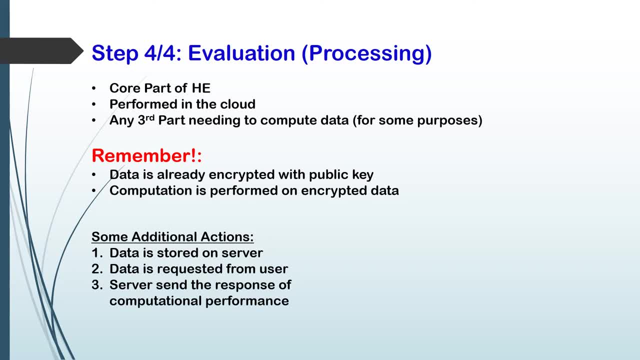 operations on the data, or it can be the end user who wants to have access to the plain text. and third one: the server sends the response of some computational performance back to the end user. the user says that hey, i want to perform some data, i want to perform some operations on my data. 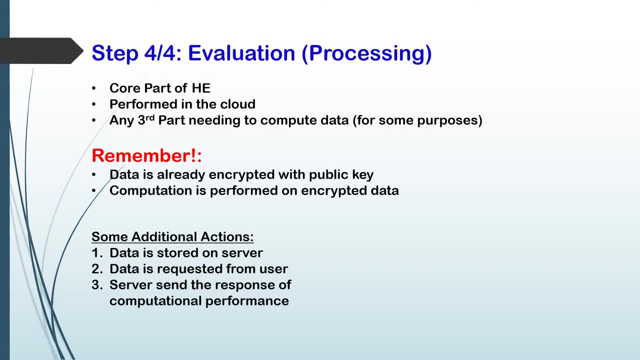 can you do it for me? the server says, yes, i can do it. send me the encrypted form. the user sends that encrypted form server performs some you useful computations, some useful operations, and sends the result back to the user. the user then decrypts it and uses it. now, as we have discussed the operation, now we will. 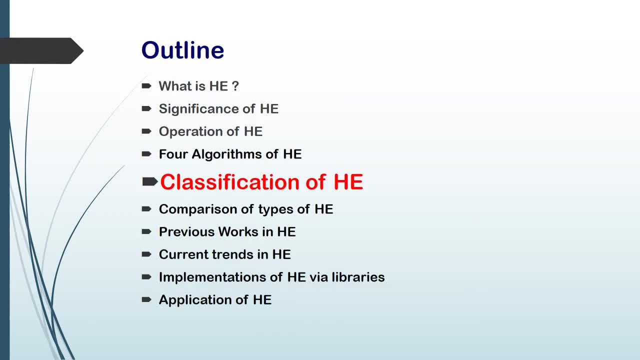 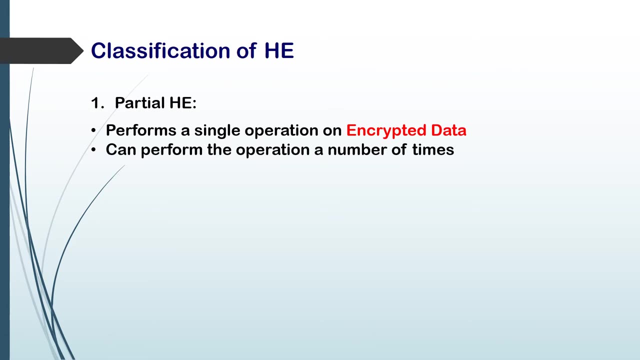 discuss the clarification. how many types of homomorphic encryption are they basically and how do we define them? now? the first is what we call something as phe or partial homomorphic encryption. so partial is something that we can say that either single operation, either addition or either. 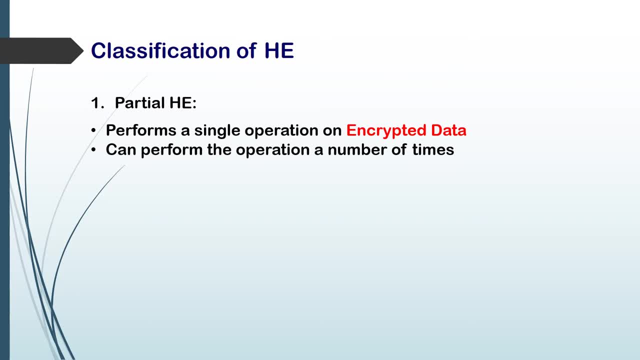 multiplication can be performed on encrypted data, but the operation can be performed a number of times. this is something to be differentiated. the single operation means that we are either performing addition or multiplication on encrypted data. we can perform only one, not two, at the same time. now, whatever operation we are performing, let's say 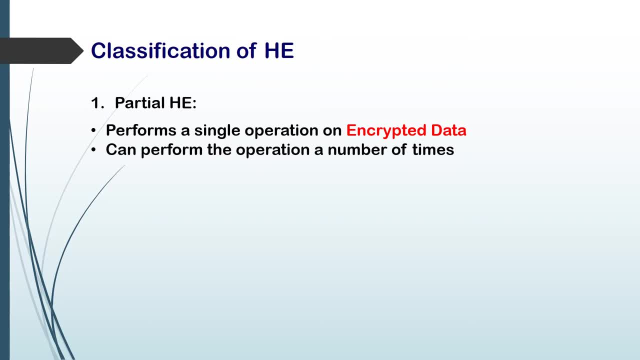 that i am performing multiplication. i can apply the multiplicative process on data the number of times i want to. this is what we call partial, because it's somehow partially. it performs operation on the data. it performs one out of two operations. now, an example of partial homomorphic encryption is well found in research papers is the helios voting. 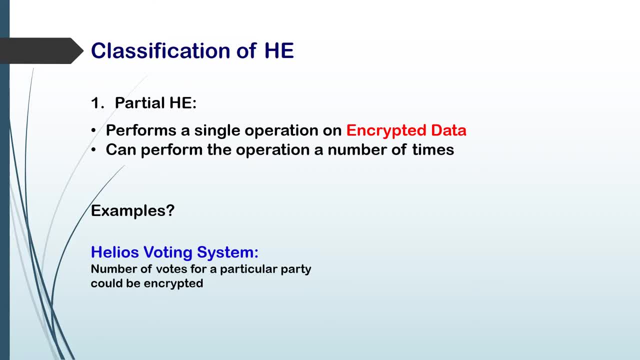 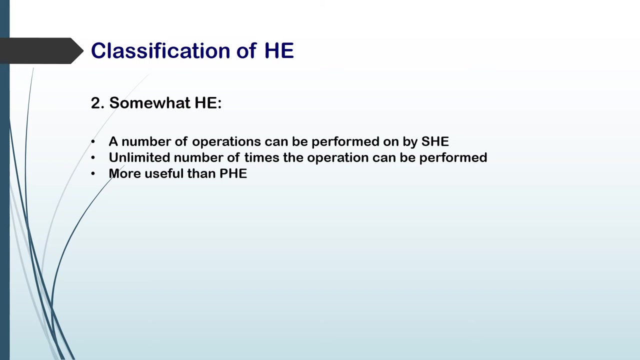 system in which the number of words, the number of words of each respective party, is encrypted so that no unwanted party, no unallowed party, can have access to the number of votes they obtained. the next time is somewhat what we call a somewhat homomorphic encryption. this is a bit further. this is one level more than the partial homomorphic encryption. 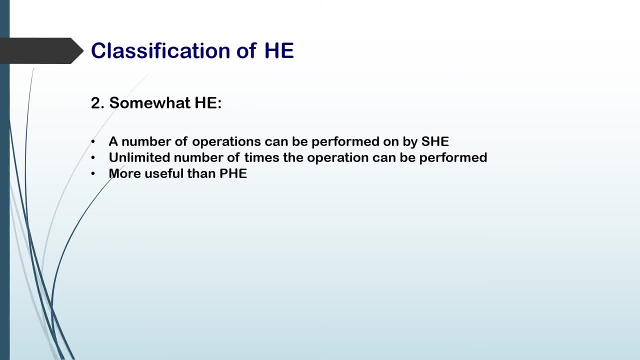 in somewhat homomorphic encryption we can perform both operations- multiple, multiplicative homomorphic encryption- and additive homomorphic encryption, both at the same time, as compared to partial homomorphic encryption, in which we could perform one operation at the time. in somewhat homomorphic encryption we can perform both operations- addition and multiplication- and we can also perform the 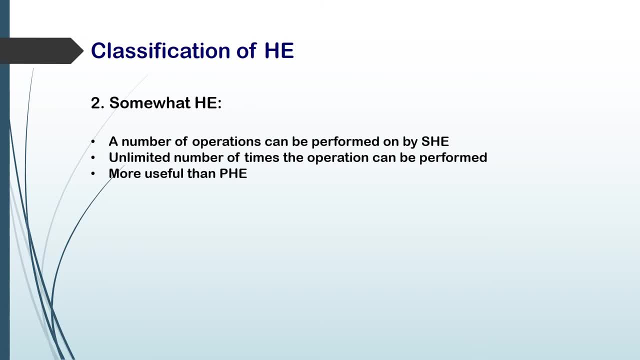 operations as many times as we want to perform it. that is why somewhat homomorphic encryption is much more useful as compared to phe partial homomorphic encryption. the third and the last type of homomorphic encryption is for homomorphic encryption, and this is one of the most powerful and the 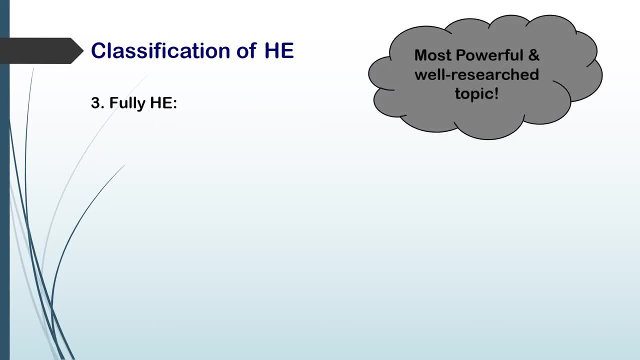 research topic in the context of homomorphic encryption. in fhe, we can perform unlimited number of operations, but only theoretically. there is always a practical limit in applying things. as we can perform unlimited number of operations, we can also perform an unlimited number of times. this is the beauty of holding homomorphic encryption. but as we all know that there are 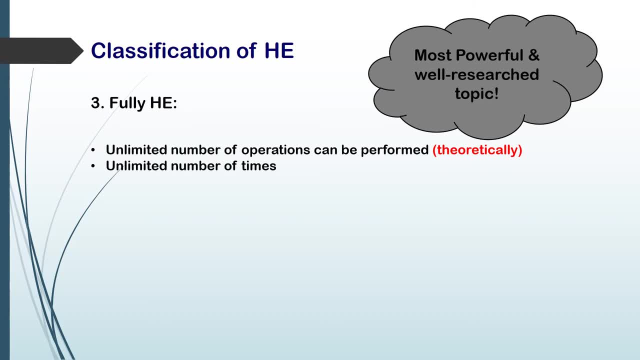 some practical limitations, due to which things cannot be applied in the same way as we expect them to be. the first concept of homomorphic encryption was developed in 1978 by three scientists, as we can see here, but the major breakthrough in homomorphic encryption occurred in 2009 and ever since there has been such much more development in fhe. in 2009, craig gentry. 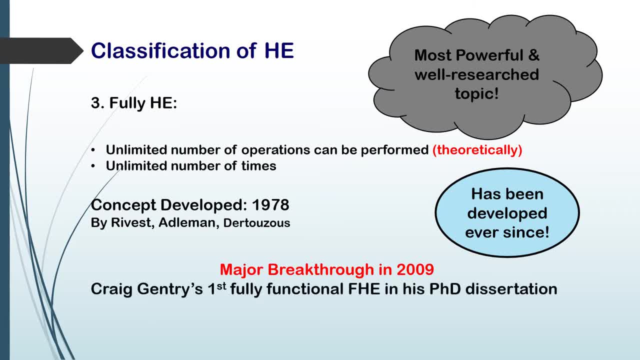 presented the first fully functional fhe in his phd dissertation at stanford university. this is one of the major breakthrough in fhe and, very honestly, much fhe much research on fhe has been based on craig gentry's f fully functional fhe. but although it was a major breakthrough, there were some problems. 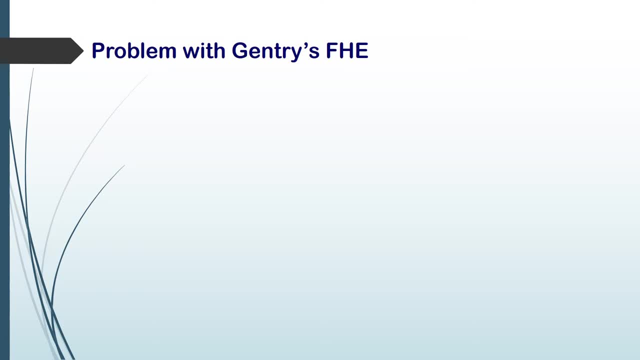 with fhe. the first of the problem that it also, although it could perform any operations, the more we increase the computations, the more errors we get, or in technical terms, we call this as noise. and this was a very serious problem in the practical field because this couldn't be applicable. for instance, let's say there are large 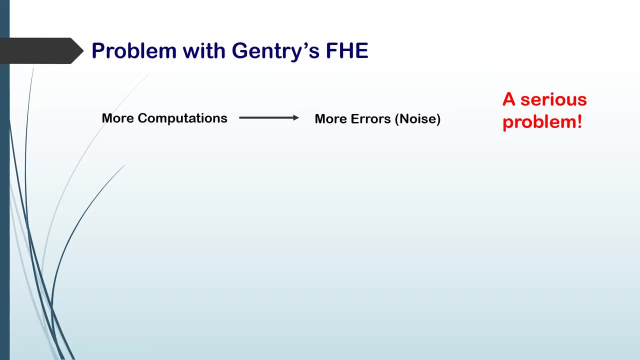 tech company wants to apply fhe. he couldn't apply it because if he increased the number of computations he would ultimately increase the errors. he will ultimately increase the noise in the encrypted data, which is more or less useless. but there was a clever solution to this, which gentry also proposed. 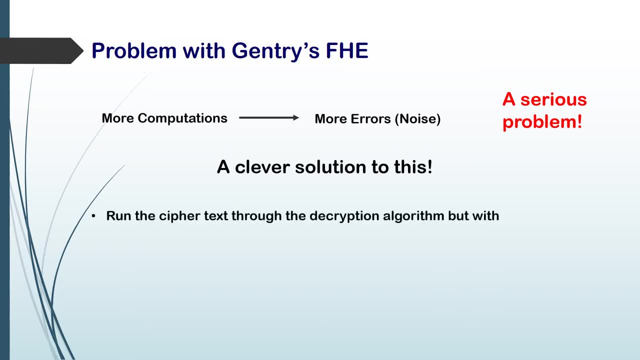 he said that let's say we have a ciphertext, we pass the ciphertext through a decryption algorithm, but with the encrypted version of the decryption key. this is a bit confusing point. we take the ciphertext and we pass it through the decryption algorithm, but with the encrypted version of the decryption. 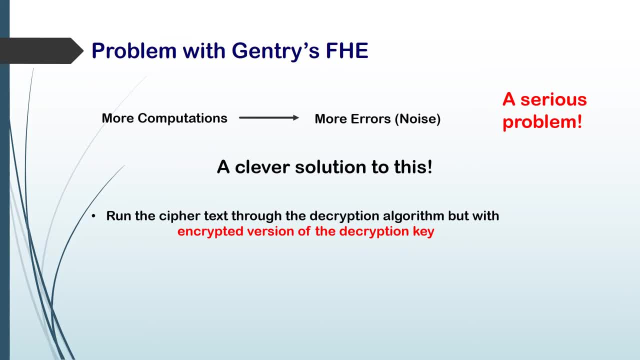 key. this is what we will discuss in a bit later. this process is actually called a squashing, in which we pass it through a decryption algorithm, but for this purpose the public key should be used and there's a also called process, which is called as refresh rate. we also discuss in a. we also 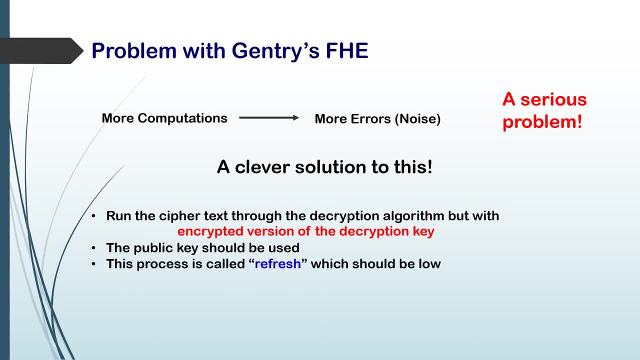 discuss in a second. what is the refresh rate? the refresh rate is a process which is called refresh rate. the refresh rate basically should be low for any practical system. the refresh rate is basically what we call of how much time it takes to develop the refresh key, to develop the refresh key for the 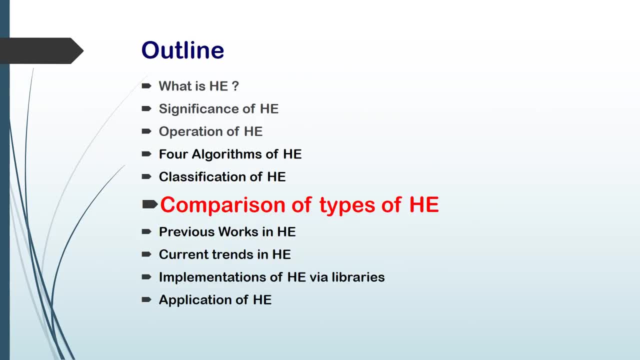 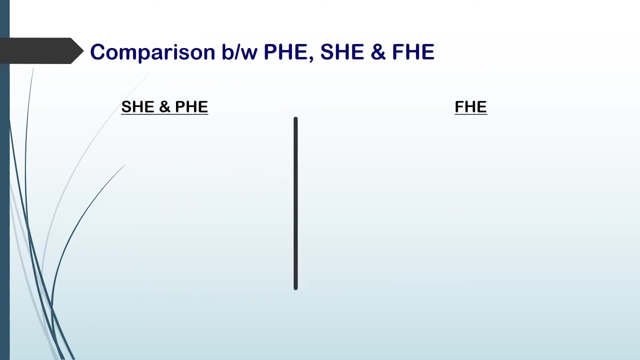 algorithm. now we will discuss a bit comparison of these three types, how these three types basically differ from each other and why do they differ? let's say that we compare types between somewhat homomorphic encryption and partial homomorphic encryption and on the other hand we have fully homomorphic encryption in case of the first part. 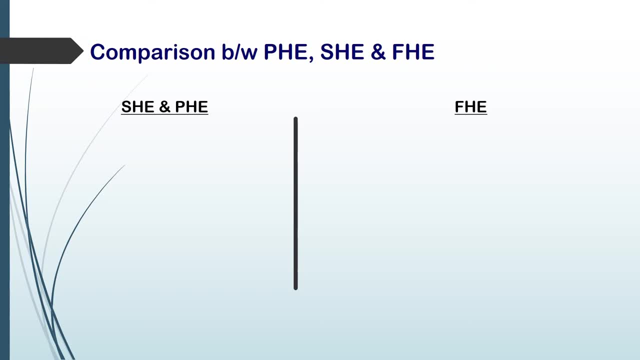 some atomic encryption and partial homomorphic encryption, we can see that they have more speed, they are faster than fhe low scale applicable and they both provide limited, limited functionality. we all know that, as we have discussed before, that partial only apply the one operation, whereas somewhat can apply both operations at the same time. this is what makes 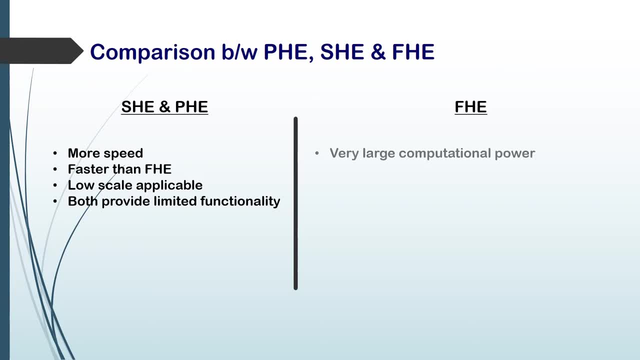 both of them much faster as compared to fully homomorphic encryption. fully homomorphic encryption requires a very large computational power because in order to apply fully homomorphic encryption, we would need to have public and private keys at a very much larger rate, which which we will discuss in a second. also, these are slower than she and phe fhe are typically not kind of practical. 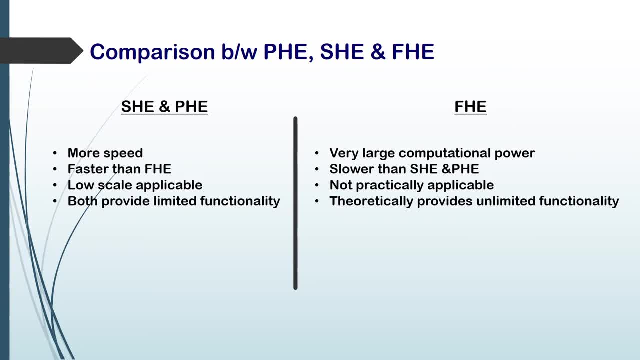 in today's, but they can be applicable if one has a lot of resources which they can apply and theoretically it provides unlimited functionality. but in theory, in literature we can see that she and phe do, although they do have low security and fhe has a greater amount of security as compared. 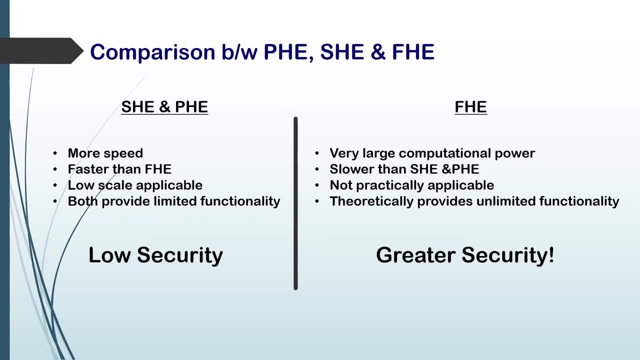 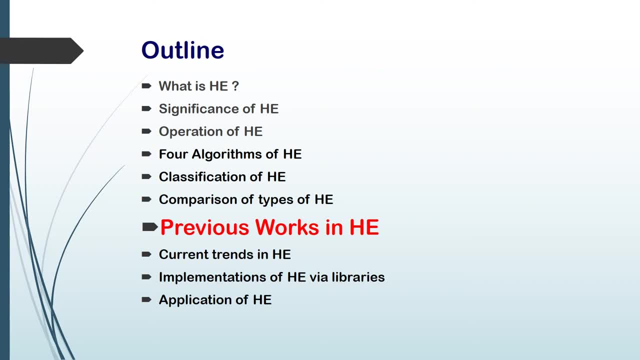 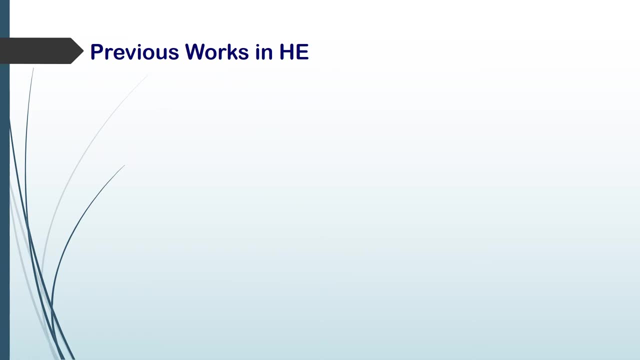 to both both of them. now let's see some previous works in he, what previous researchers have done in the context of he. first of all, i would like to discuss two main things in this context, although things can be very much complicated at this step, but i would like to keep keep things very simple. 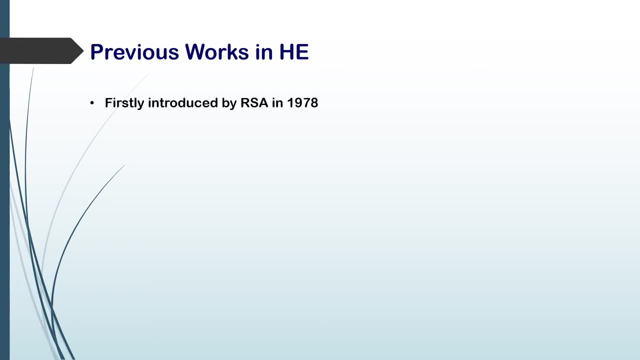 as we have discussed that the first concept was introduced by rsa in 1978 and the second was gentry's özg in 1978 and the second was Dwight Ritz uh, who was a rather internecological rival in the country and he continentalist, so he used his own fhe, aunque sônercé faisait ne façade fhe. 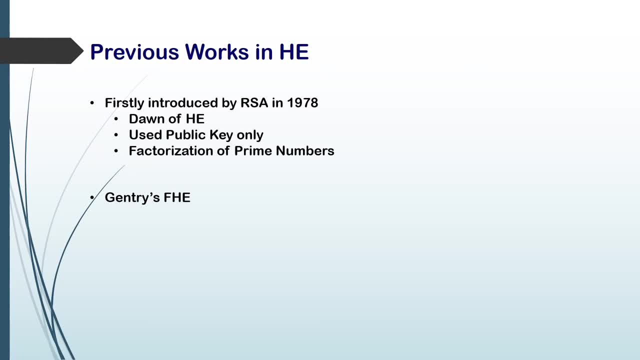 in 1978, it was the dawn of homomorphic encryption. it only used private, it only used public keys and the encryption involved in it was somewhat the factorization of rhyme numbers instead of using any standard election, for example, doubling an input of the prime numbers as the encryption key required for the encryption in gentry's fhe. 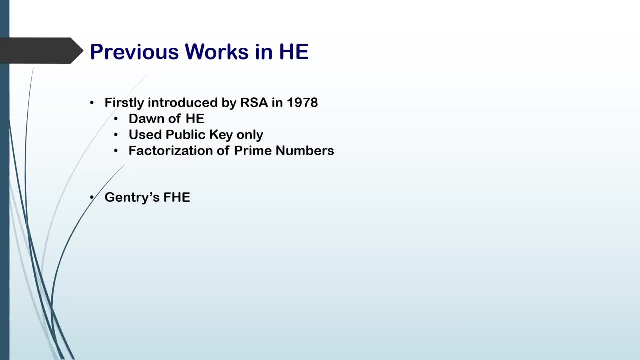 gentry basically applied a very clever technique to generate fhe. he didn't directly generate it, but he indirectly generated it. he converted somewhat homomorphic encryption into fully homomorphic encryption. he used a technique called as bootstrapping. bootstrapping is basically when we convert she into fhe. this is what we call bootstrapping and this basically defines the. 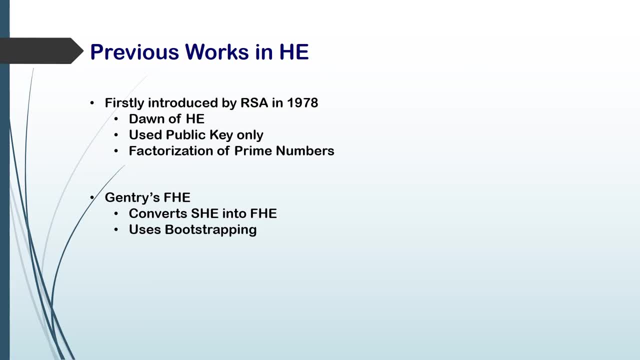 extent of gentry's fhe. the more bootstrapping you can do, the more applicability you can achieve with fhe. and gentry applied his technique. he is fhe based on lattice algebra, which is a discrete mathematics, which is a discrete mathematics subset. now i would like to discuss that how basically fhe is implemented in theory. first of all, we 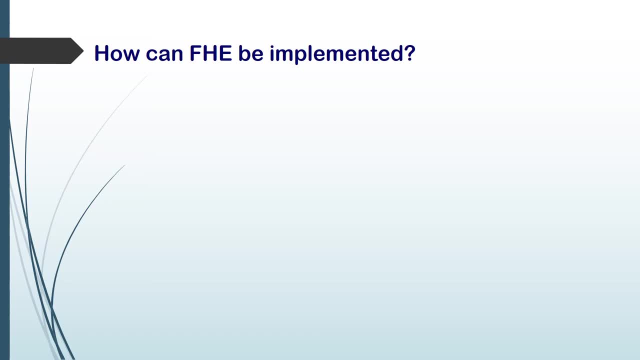 as we discussed before and gently also apply to it, that fhe can be implemented by lattices, but lattices had a major disadvantage is that they produced a public size key of approximately equal to 2.3 gb, which is a huge amount. this is not a 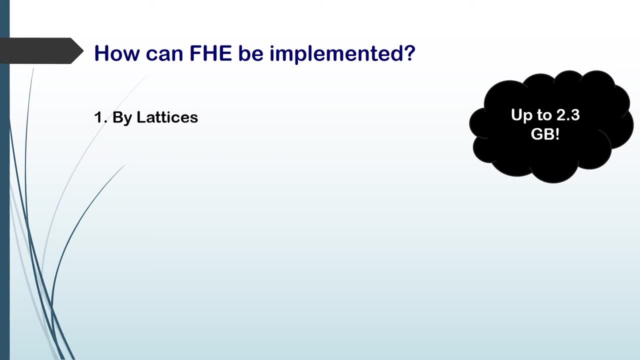 applicable practically on a very large number of users. lattices had this major disadvantage. the second type was integer base and the third was ring learning with errors. these are basically very complex topics in discrete mathematics which can be studied individually, but we are not going to discuss it here because there are very complex topics and they can. then i cannot be explained in. 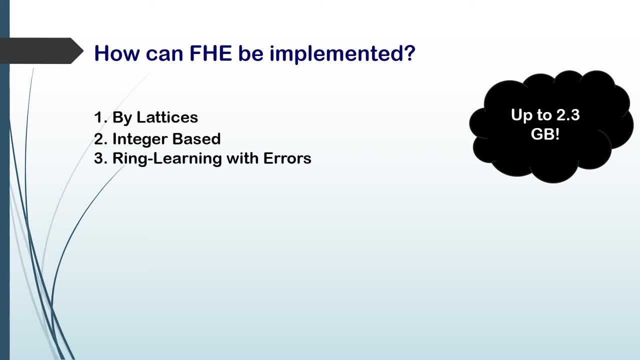 a very minute amount of time, so we will discuss our. we will discuss our topics one by one and we will see, first of all, what is mean by lattices. by lattices we mean lattice algebra. this is also a basic subset, as we discussed before, that this generated. 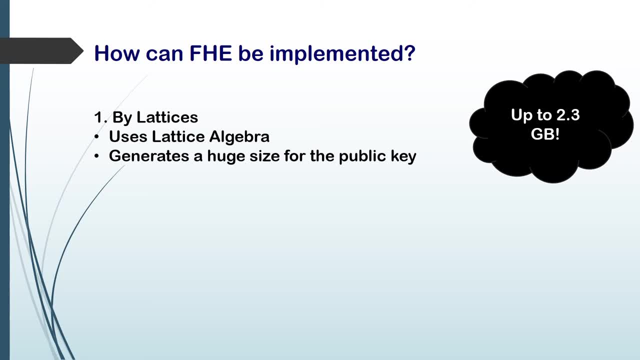 a huge size for public key which is not physically applicable because we have a large amount of users. a number of researchers tried to apply fhe using lattices, relatively with a small amount of, with a small size of FHE, but it didn't go very well. 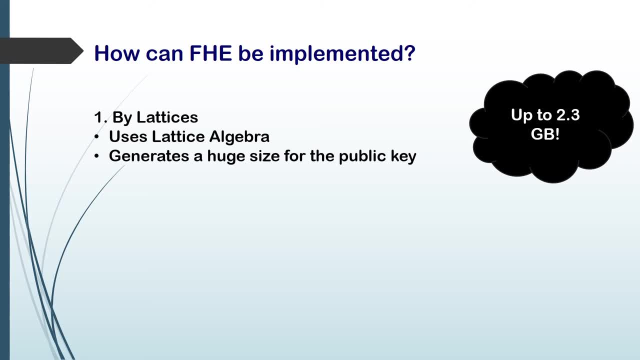 there were some disadvantages with lattices, for instance. let's say I have attached the references below. in that references the paper number one: it implemented FHE using lattices on a core i7 at the rate of 3.4 GHz and 32 GB of RAM. 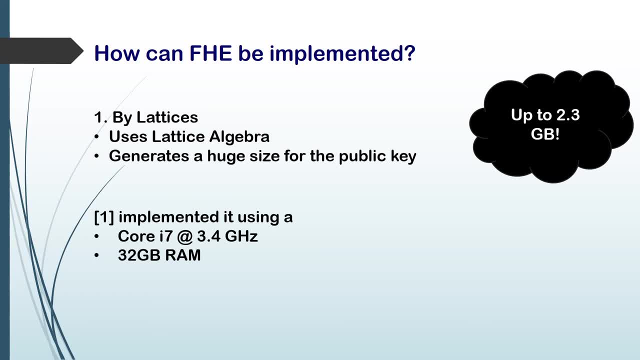 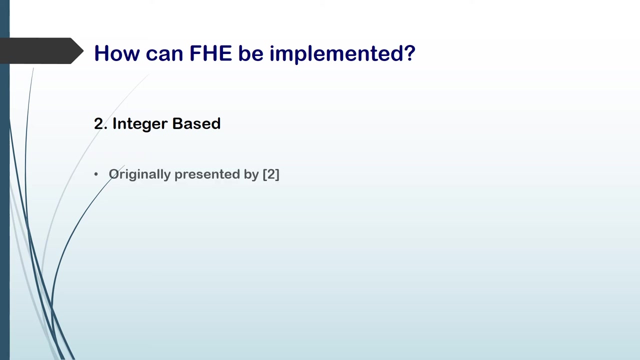 but this produced a public size key of a whopping 5.6 GB, which is a very huge amount. this cannot be applicable. this cannot be applicable practically. the second thing we can see: integer based. integer based, it was particularly produced by the authors of reference to paper number two and similarly a number of 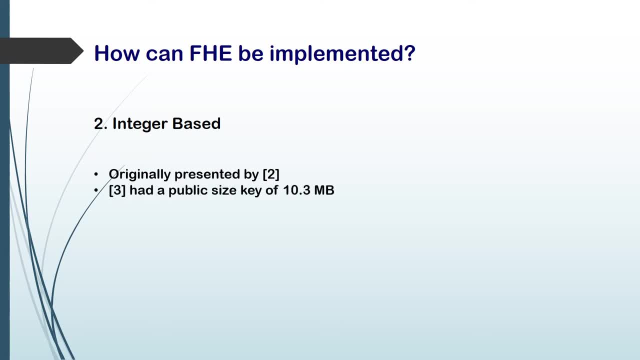 other authors have also presented it. we can see the reference paper number three. he produced a public size of 3.3 MB which is very much applicable. but three was a bit modified version of paper number four. all of these paper I have attached in a separate 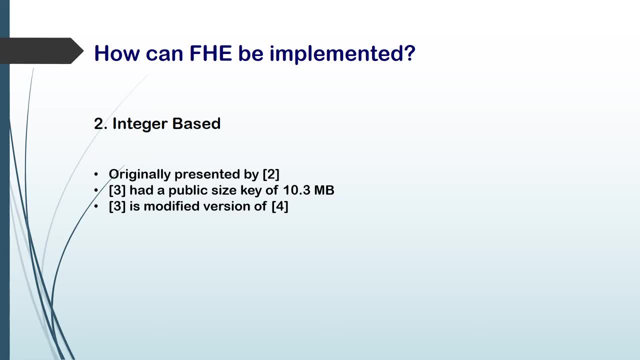 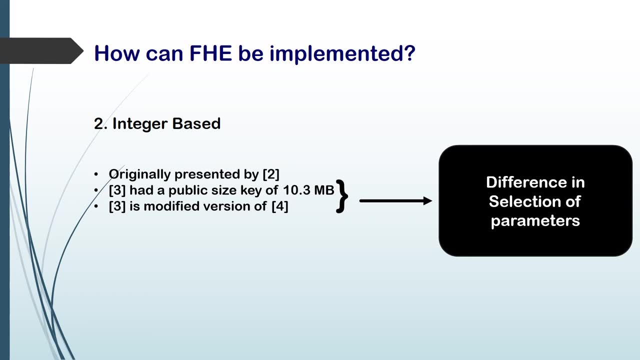 file below, you can see them. the difference in these two was basically of the selection of the parameters. they use different parameters to select in order to perform their encryption, and that is what makes this 10.35 MB. and the third is learning ring- learning with errors. this is also basically modified. 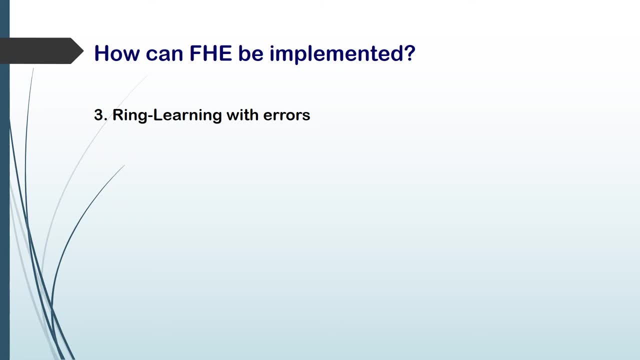 version of learning, with errors. we can say that a bit modified version. it was originally presented by the author, the paper number five. also it had a bit positive point. that the solution of this can be reduced to the hardest of lattices means that up till the extreme which lattices can be formed. reclining can produce those solutions very easily. 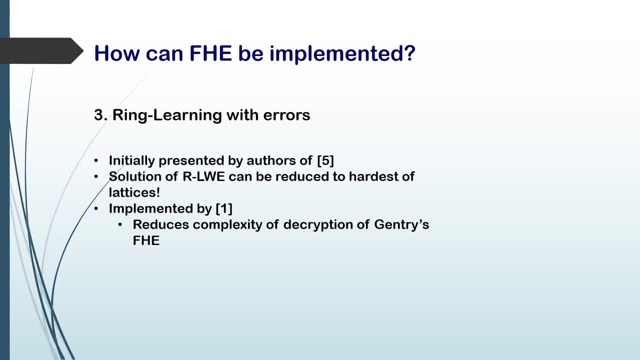 It didn't have a very much hard time. It also implemented by the paper number 1. It reduces the complexity of Gentry's FHE, which is also very much applicable in some practical point of view. We all know that all of these three types have some scalability and limitations. 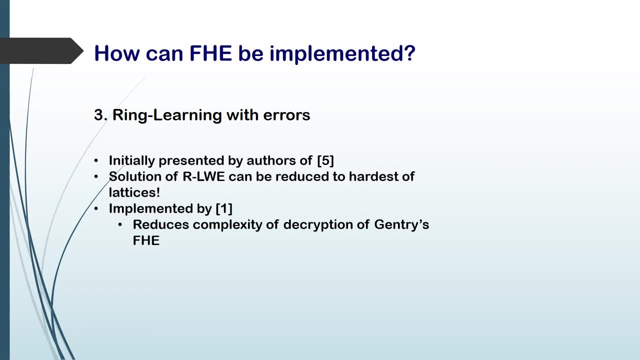 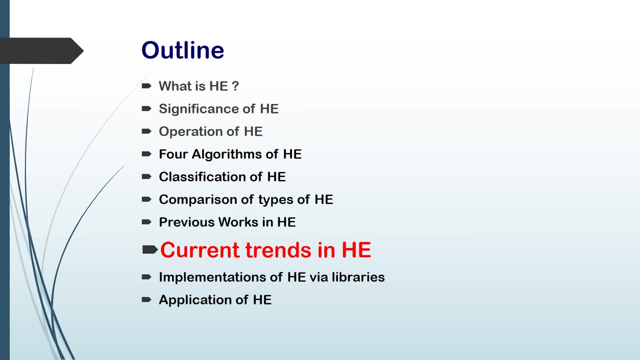 And which method you apply. all depends upon your necessity, all depends upon your requirement of what you are basically requiring. Now, as we have discussed in previous works, we will discuss of some current tense. What are basically the current tense of homomorphic encryption? 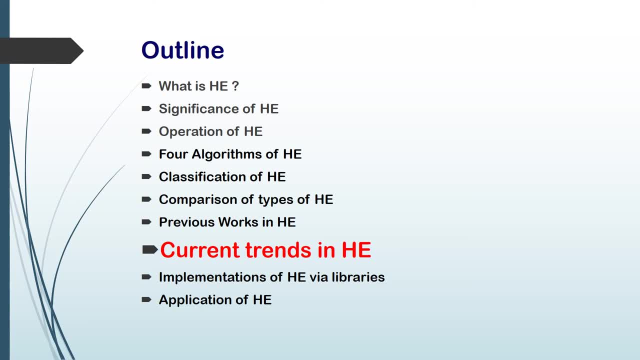 What is happening today in the domain, What is the domain of homomorphic encryption? First of all, before discussing very specific, before considering each specific example of current tense, I would like to discuss a very few common things which are also presentable in this context. 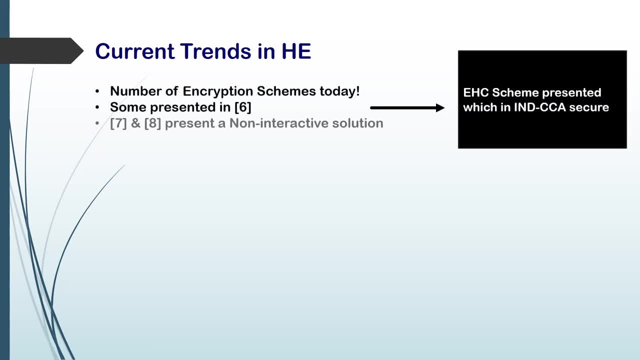 First of all, there are number of encryption schemes that are available today. Some of them are presented in 6.. In the site description box we can see that EHC scheme is presented in paper number 6, which is INDCCA secure. I would like to discuss a bit detail on this. 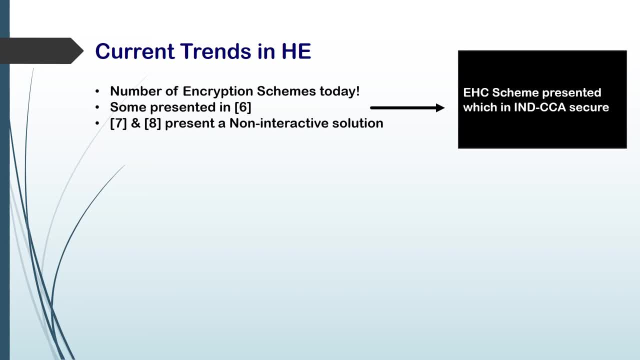 Basically, INDCCA is a new type of homomorphic encryption. It basically uses a concept as we discussed before, but in a new way. INDCCA is basically an other objective of cyber security field. We discussed the first one, that is, CIA, before at the start of the presentation. 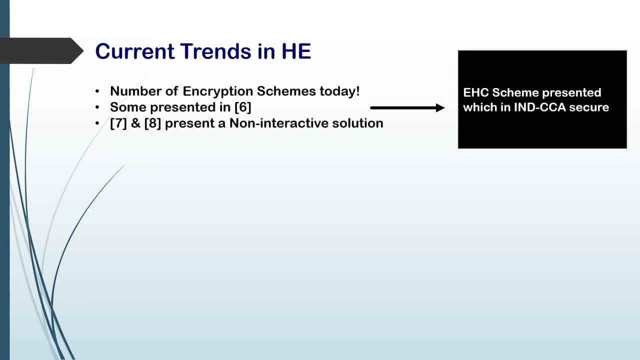 INDCCA is another objective that we can also obtain in the context of the cyber security field, Or in specific, if we say we can see that it can be applied in the context of homomorphic encryption. Basically, 7 or 8 papers have also 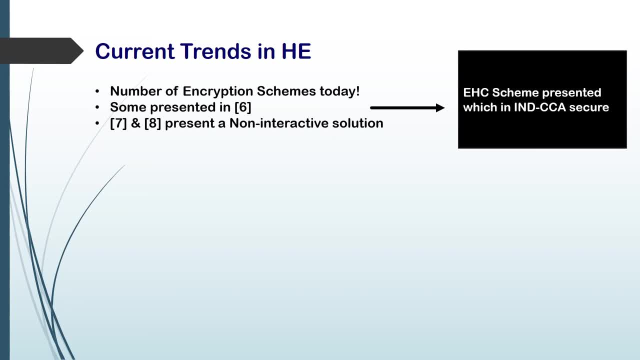 discussed some non-interactive solution of homomorphic encryption. Now we will discuss a simple general scenario of how this actually works. Let's say that we have two users: Alice and Bob. Alice has some data that she wants to perform an operation on. 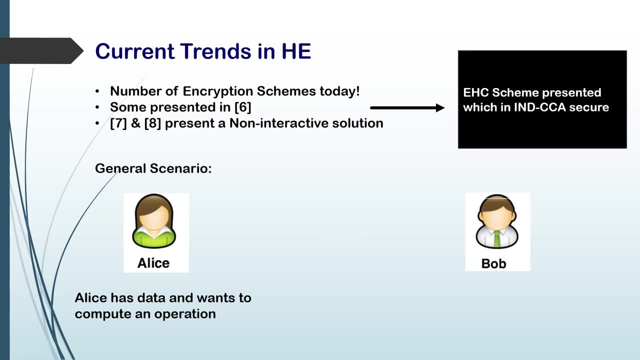 But the problem is she doesn't have any resources to perform that particular operation. She comes to know that Bob somehow has the function that can perform the operation on any type of data. So Alice also doesn't want to share the data in plain text form. 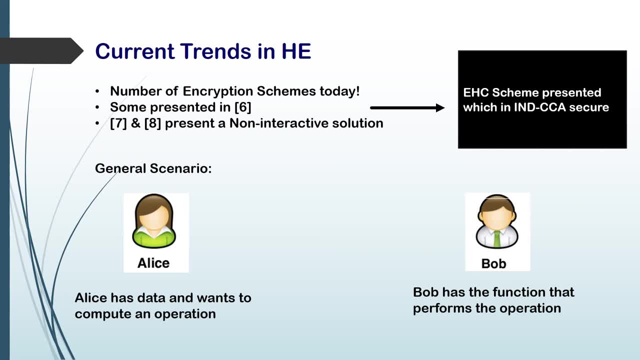 So Alice sends the data in encrypted form to Bob. Bob receives the data, performs an operation and sends it back to Alice. Alice then decrypts the data and performs the necessary operations if she wants, Although the operations were performed by Bob. if there are some simple applications that she wants to perform, 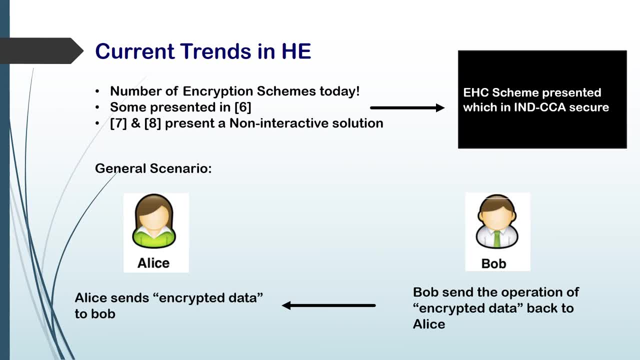 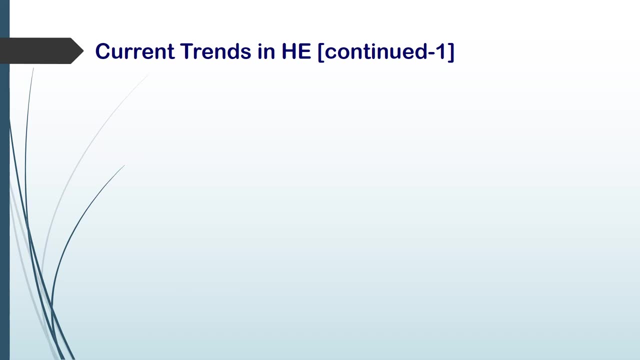 she is easily available to perform it. Now let's talk about some specific examples in the current trends. First of all, I would like to discuss here that machine learning is also stepping in in the field of homomorphic encryption. Let's see. 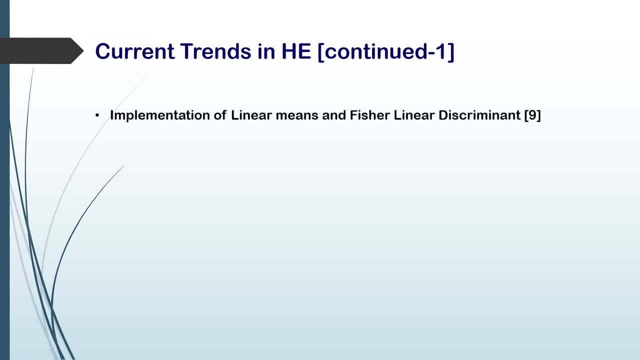 The authors of paper number 9,. they implemented linear means and Fisher linear discriminant in homomorphic encryption. Basically, these are two algorithms in machine learning that are applied to homomorphic encryption. This can also be viewed at paper number 9.. Another author has implemented neural networks on encrypted data. 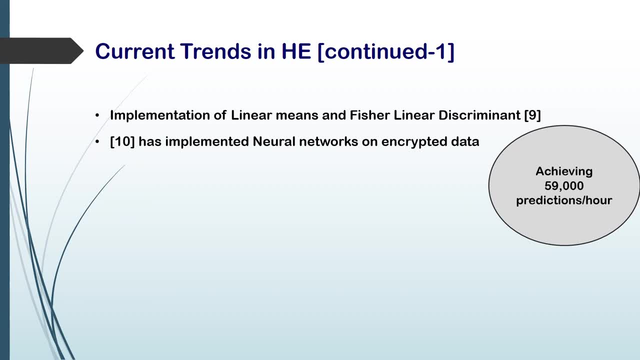 which was achieving 59,000 predictions per hour. This is also a major breakthrough, But the problem with this is the same: that it cannot be applied at a major scalable at a very large level. The next presented some logistic regression using various homomorphic encryption schemes. 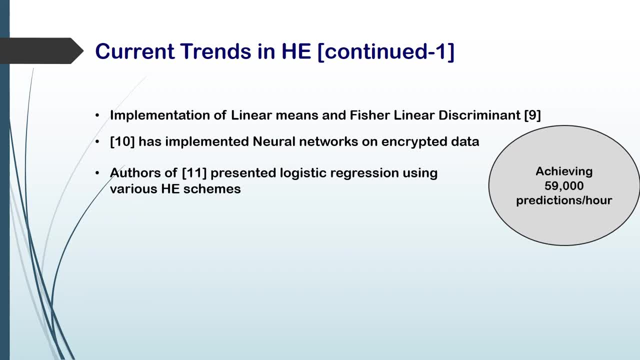 They used only additive homomorphic encryption- And also their work, which means the authors of 11,. they were based on the work of Pellier, LWE, Ring Learning With Errors and Ring Learning With Errors along with Simple Learning With Errors. 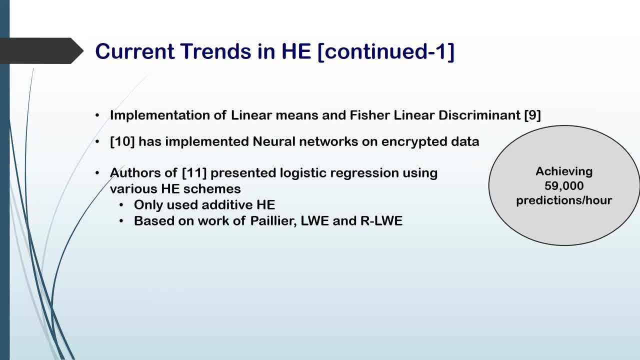 And the next. they applied homomorphic encryption, they applied homomorphic cryptosystem or, in other words, the same thing: homomorphic encryption to facial recognition. This is also a very major application of machine learning in the context of homomorphic encryption and vice versa. 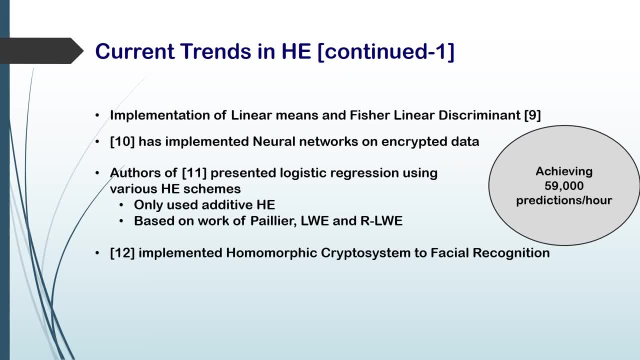 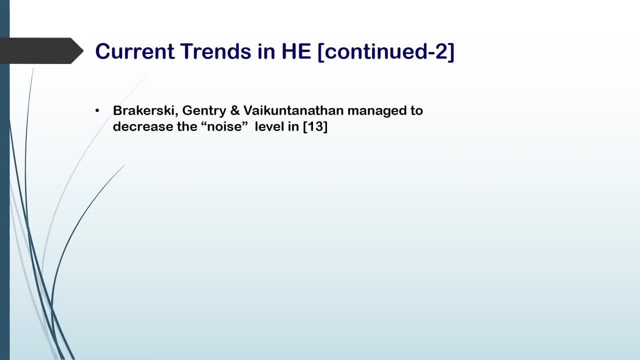 Similarly, we can see that there are a number of others, other homomorphic encryption that are also presentable. Gentry, along with two other scientists somehow presented, somehow managed to reduce the level of noise that was originally produced in Gentry's FHE scheme. 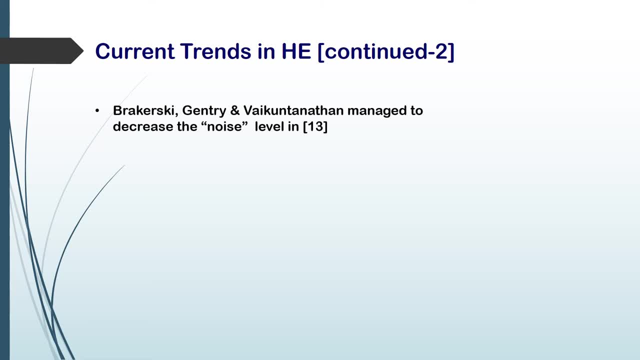 They presented their work in paper number 13,, which can also be seen anytime. But how did they manage to do it? This is a very clever technique also. They, instead of increasing the addition in multiplicative operations, they rather increased exponentially. 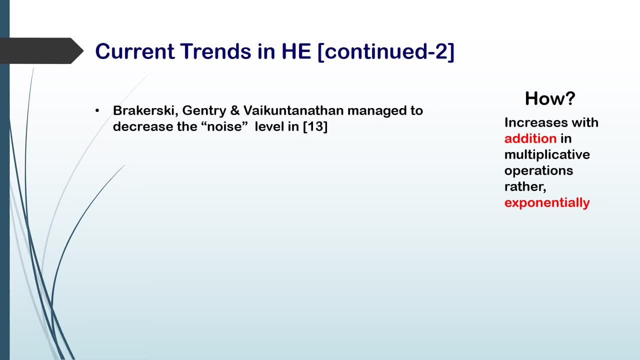 which means that, instead of as soon as the multiplication operations are increased, they are not increased exponentially, but they are increased additionally, which means that, for instance, let's say that we are performing three multiplicative operations, so three additive operations will also be performed. 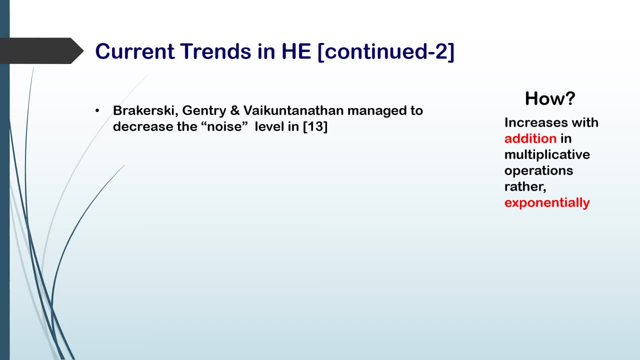 This is the range in which the noise will be increased, instead of exponentially, which was previously being generated in Gentry's original 2009 scheme. And another very important major breakthrough in the context of FHE is the application of homomorphic encryption and quantum technology. 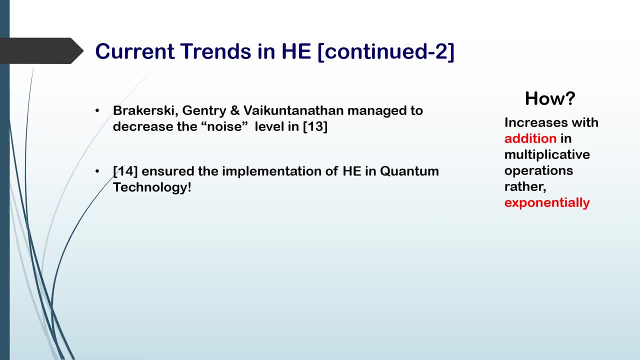 Quantum technology is a very major, is a very hot field in today's modern era because most of the computing, most of very large industries are trying to perform quantum technology. They are trying to produce quantum computers because they have very large capacity as compared to today's traditional computers. 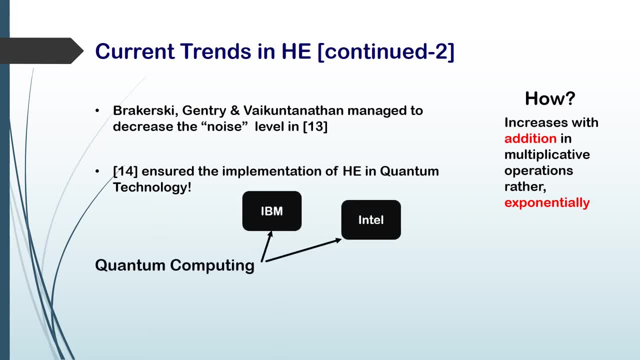 Some of the quantum quantum computings. IBM is performing quantum computing, Intel, Microsoft, Google Quantum, EILAB. These are some of the very famous industries that are performing quantum computing And these operations, these operations that are performing. 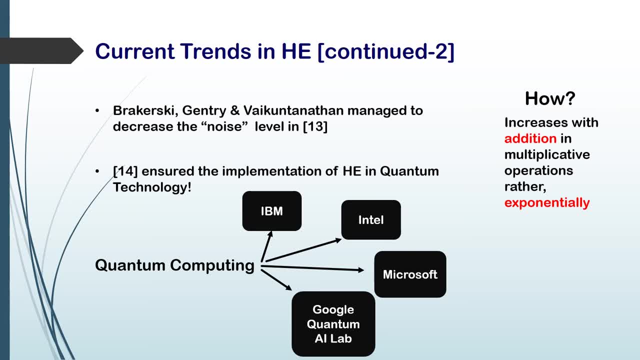 they are also using FHE Up to some extent. this research is still under consideration, It is still under the process of research. Now, after we've seen the current trends, current trends in homomorphic encryption, we would like to see that. 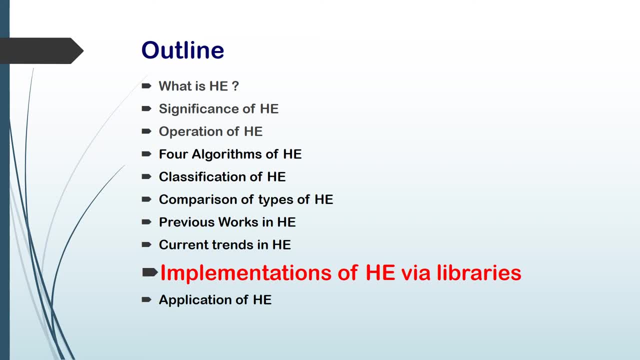 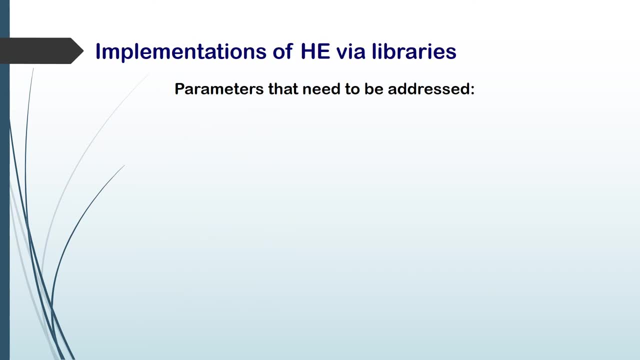 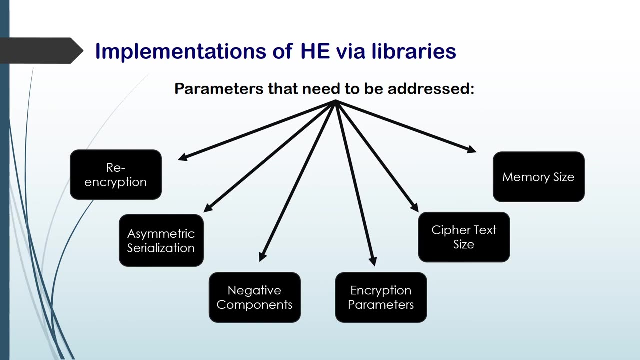 how is it implemented via libraries? But before we discuss it specifically, I would like to discuss some of the parameters that need to be addressed in order to understand how it is applied via a library. Some of the parameters that can be addressed are: re-encryption. 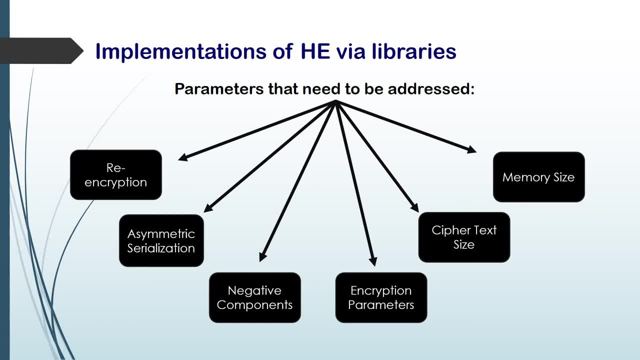 asymmetric serialization. negative components: encryption parameters, ciphertext size, memory size. Each of these parameters are visible from their names. what they exactly do. Re-encryption is the method of performing again encryption on serial data, performing again encryption on ciphertext. Asymmetric serialization is somewhat. 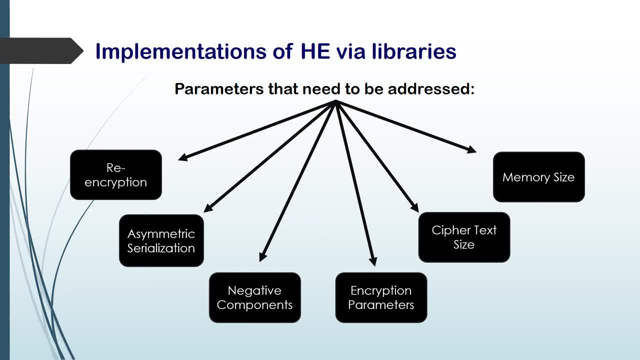 it's a difficult thing to understand So I won't be able to discuss here, Although it can be easily searchable from net. It can be easily searchable from the internet. It is a very certain topic to understand. Negative components is also. 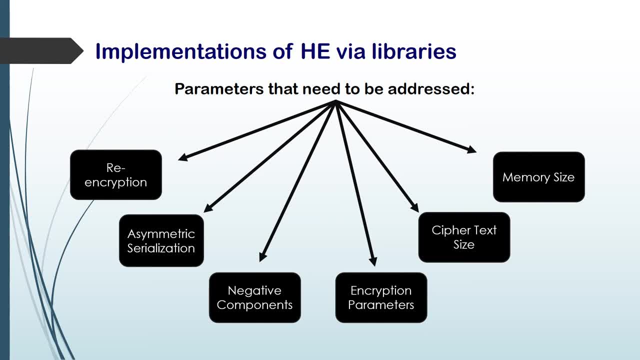 when we introduce negative parameters into the encryption instead of using positive, always all the time Encryption parameters. these are also very few things that we have to discuss. Ciphertext size: obviously, as we discussed previously, the ciphertext size has to be manageable in order to understand. 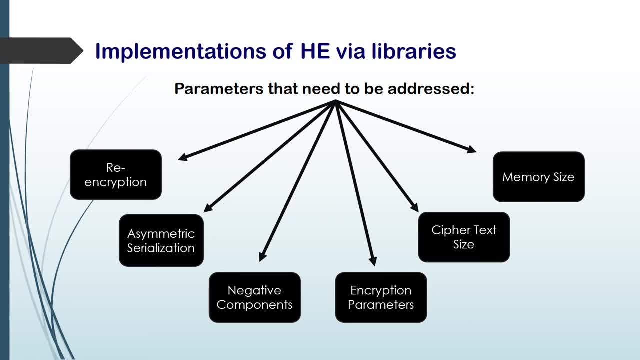 to apply homomorphic encryption at a practical level. Memory size: it also depends there. Memory size also. it depends upon various parameters. Memory size is basically the amount FHE requires in order to perform its basic necessity operations. Next we will discuss a few libraries. 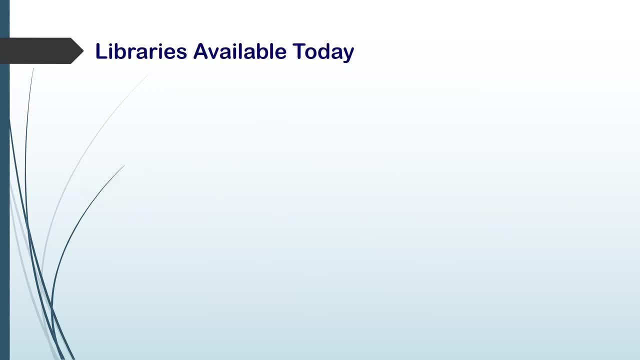 where homomorphic encryption can be applied. Out of those many libraries, some of the most famous that can be used are Microsoft SEAL, Pyfell and HeLib library. Microsoft SEAL as its name. it was originally presented by Microsoft. Its current version is 3.5. 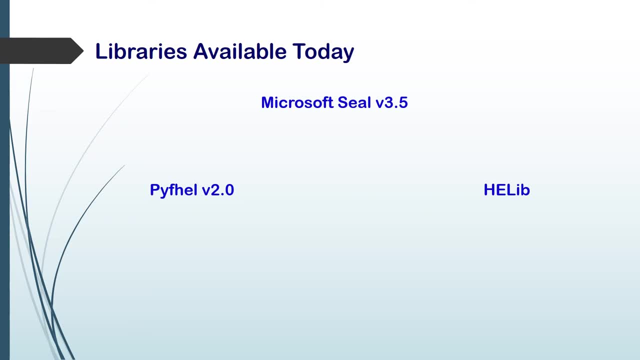 It has been developed since version 1.0.. It can be implemented in Microsoft Visual Studio 2019.. Basically, it applies two kinds of schemes: BFE and CKKS. These are basically two types of schemes. What we mean by homomorphic encryption scheme. 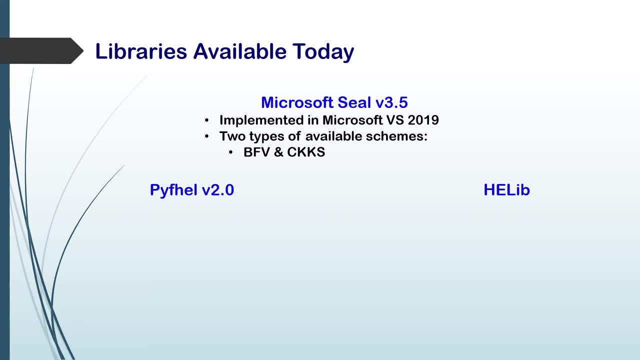 is that it performs addition or multiplication in a very specific way that it differs from other encryption schemes. Basically, this is what we call an HE scheme. It's nothing else. Pyfell is a Python library and its latest version is version 2.0. 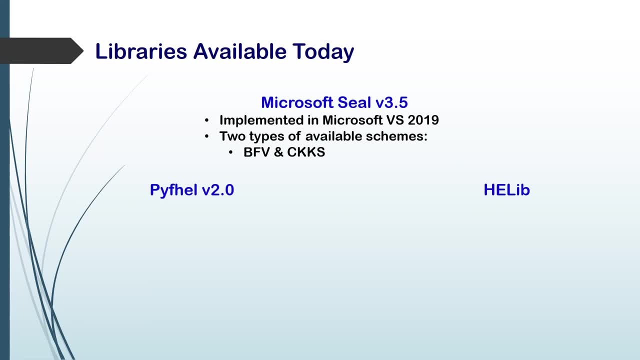 Pyfell library is basically a library that you can download and operate on any type of a computer with large computing power. This is the only condition You have to have required very large computational power. It allows submission, attraction, multiplication of encrypted data. 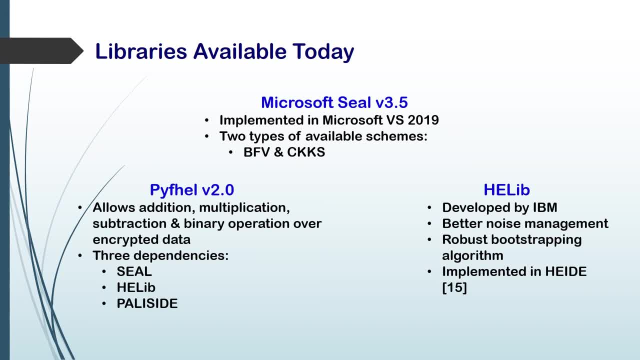 It depends upon three dependencies: SEAL, which is Microsoft. SEAL, as we discussed. HeLib, which is also, And Pyfell, It is also another library using homomorphic encryption. HeLib was first developed by IBM. It has better nodes management. 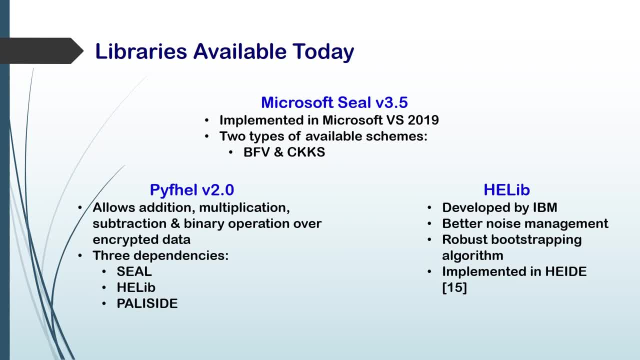 It has robust power bootstrapping algorithm And it is implemented in HE IDE. This is the IDE used for HE Lab And this can be found in paper number 15, which I have attached below. These were some of the major libraries that can be used. 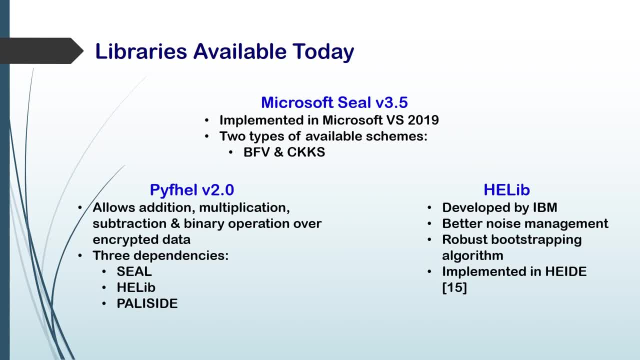 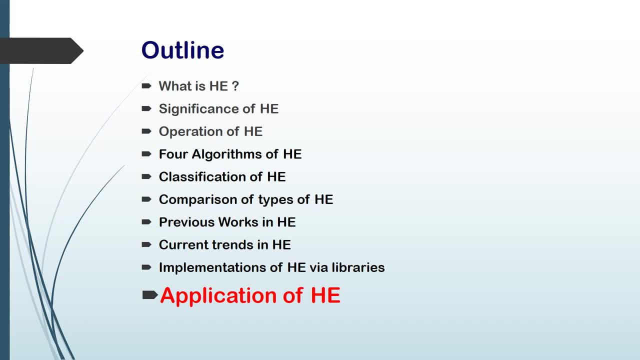 in context of homomorphic encryption. Next, we have application of HE. This is the most important part of this whole entire presentation is that we discuss where can homomorphic encryption actually be applied, But not least, applications of homomorphic encryption, As we have discussed. 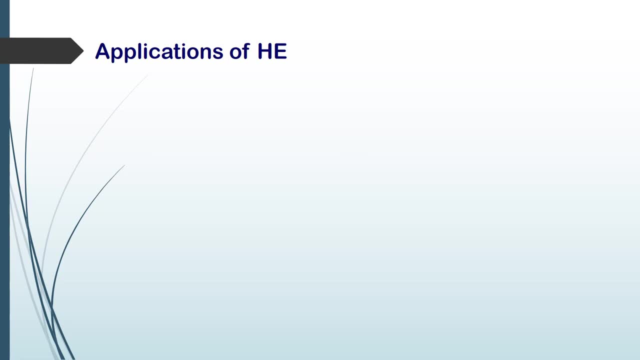 homomorphic encryption has a number of applications, But the only problem we lack is that its performance. It cannot be fully applicable at any stage, But we will still discuss some parameters, some applications that are worth discussing. First of all, bank transaction. 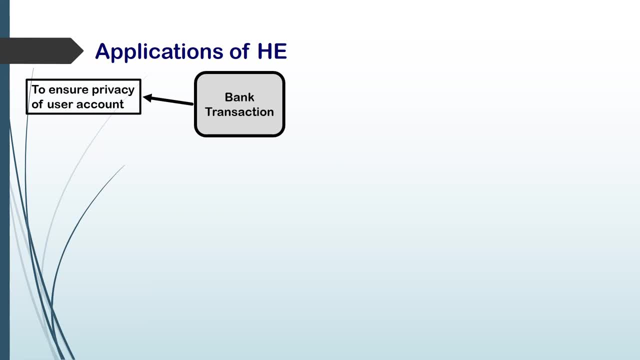 Bank transaction is something to ensure user account privacy, user account data. It is very clear from its description as well. Control system is something that we can use to protection of the sensor. Sensors are some real-time physical devices that sense the environment and report back. 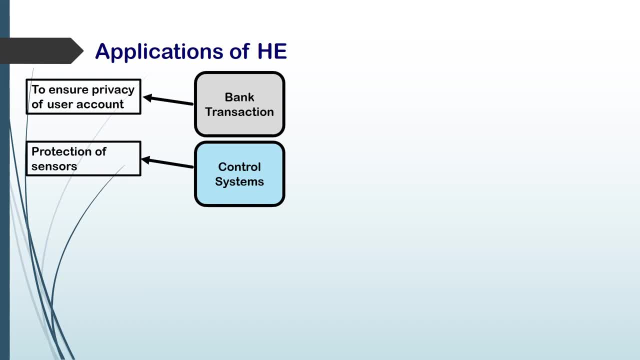 to a computer node. In order to protect the data that travels between the node, that travels between the sensor and the main part, you can use homomorphic encryption so that it cannot be used by any other third party, unwanted third party. The third is cloud computing. 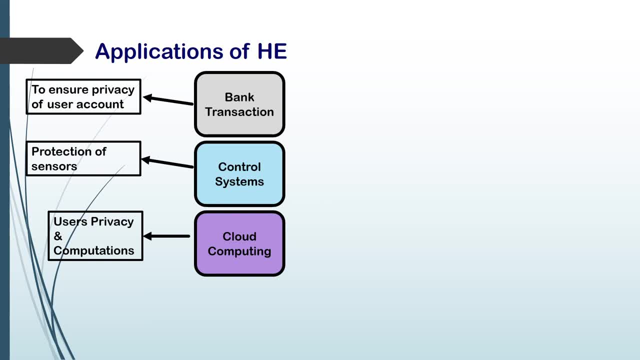 This is also a very major application In cloud computing, as cloud computing is also evolving. homomorphic encryption can be used in cloud computing to ensure that user privacy is the first and foremost priority, as well as its computations. These are also very important applications. 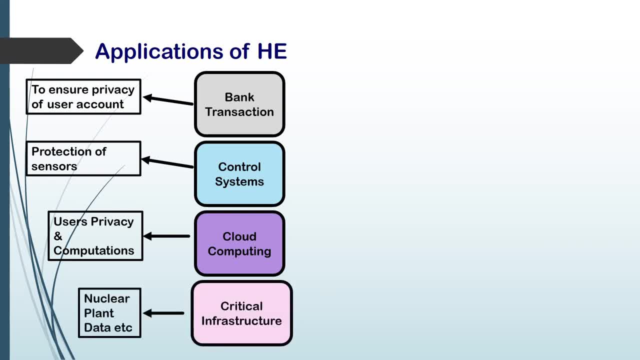 Fourth, one becomes the critical infrastructure, such as a nuclear plant data. For example, if there is a nuclear plant developed in any part of the world and it develops data which is required to be encrypted, instead of using encryption- data encryption- we can use homomorphic encryption. 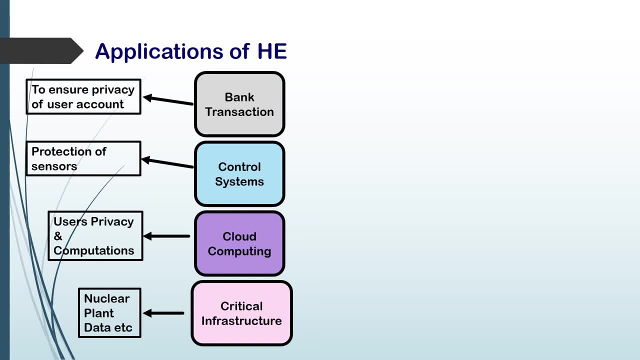 which increases the level of the encryption as compared to standard encryption. WS and wireless sensor network: This is also a very emerging topic. This is where production of nodes come into place. Wireless sensor network, as the name suggests, is a network consisting of sensors deployed at different locations. 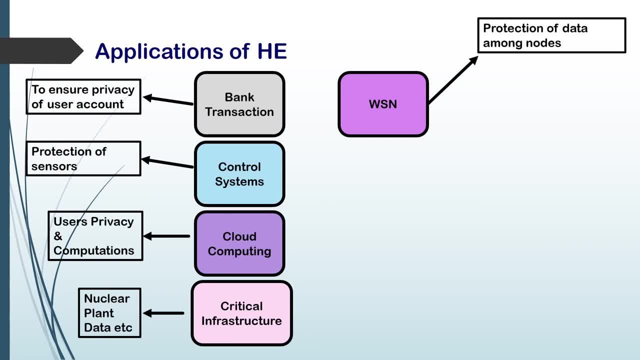 at a specific area In order to put data among the nodes or any other, not just data, any control message, any specific message between the nodes. we can use homomorphic encryption, Search engine optimization. This is also a very interesting application, For example. 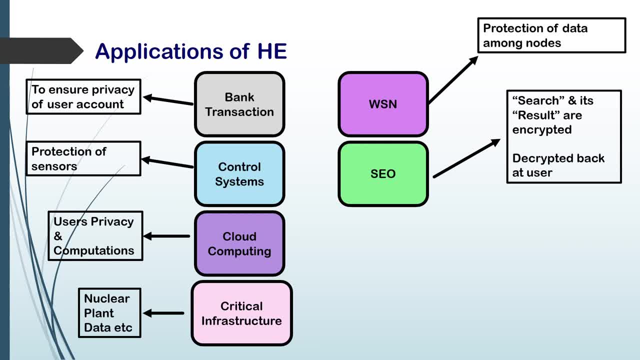 a user wants to search for some query, but he ensures that he wants his search to be encrypted. The search and the result: both are encrypted. The search engine, whoever it is it, operates the search based on the encrypted data and then sends the necessary result. 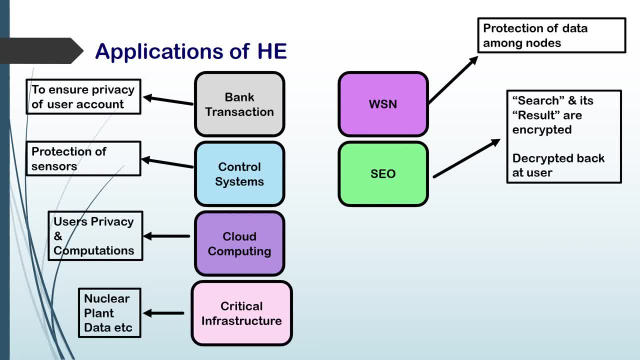 back to the user in encrypted form. The user then decrypts it and then it is presentable in a usable manner. Similarly, as we discussed before, e-voting system is also another very important to ensure privacy of the respective parties. No unwanted party can access. 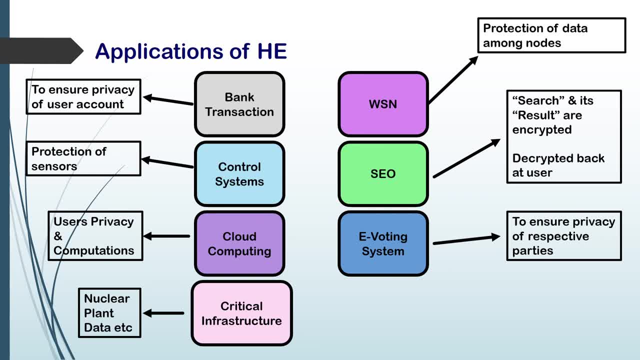 number of votes of any other party. on big data, For example, this is a very specific CERN, the European Organization for Nuclear Research. This is produced 75 petabytes of data in 2010 to 2013.. This is a very large number. 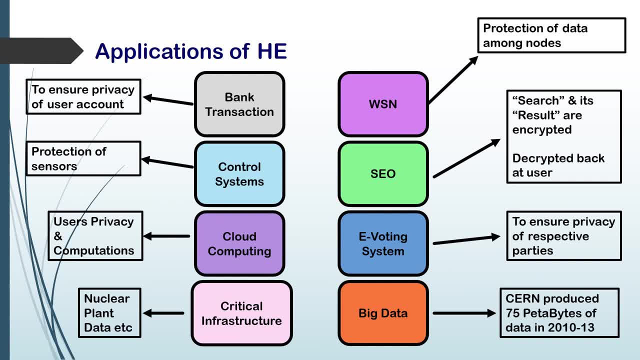 75 petabytes in 2010 to 2013.. This also contains very sensitive data that can't be released into the public until very much processed. For this data encryption, homomorphic encryption can be very much used. Next we have the 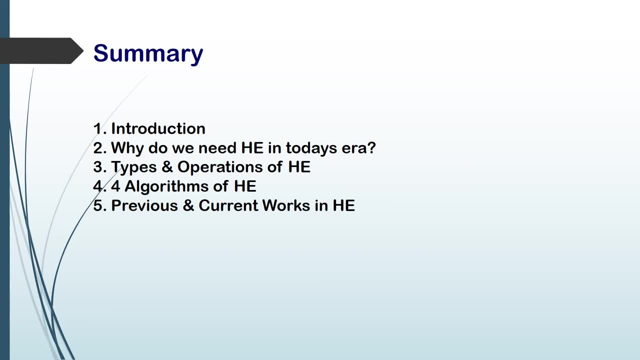 four-fold summary of our presentation We will discuss: we simply discuss introduction to a chain. what is a chain? why do we need it in today's era? we discuss its importance. Sony PlayStation 11 hack. Aquafix 2007 hack. 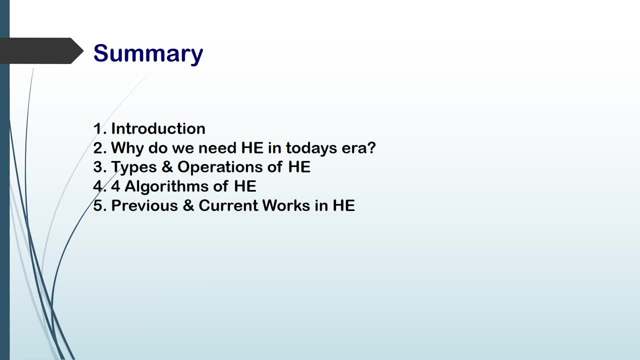 we discuss the types and operations of homomorphic encryption. we discuss what are the four algorithms in homomorphic encryption, previous and current works in homomorphic encryption. Thank you everybody for watching this presentation And if you need any more detail, you can feel free to contact me.